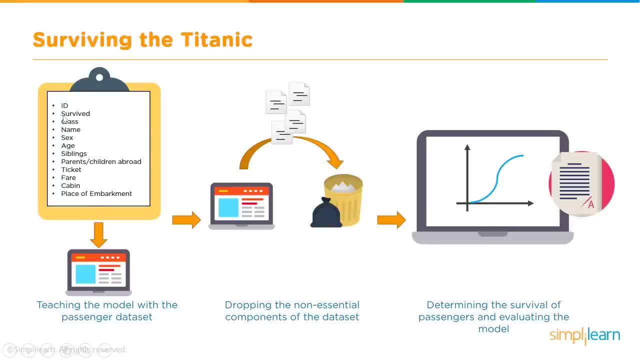 the non-essential parameters or attributes. here We only take those attributes which are really required to make these predictions, And once we train the model, we run new data through it whereby the model will predict whether the passenger has survived or not. So let's see what. 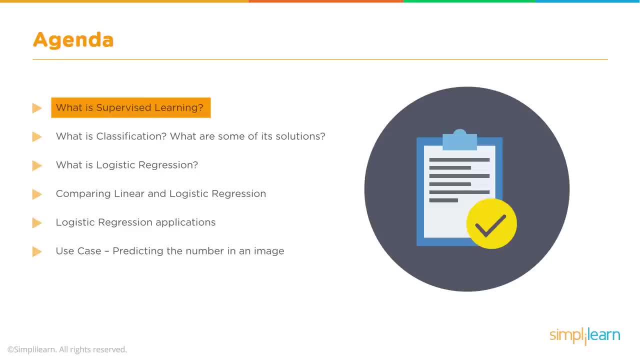 we will learn in this video. We will talk about what is supervised learning and we will go into details about classification, which is one of the techniques for supervised learning, And then we will further focus on logistic regression, which is one of the algorithms for performing classification, especially binary. 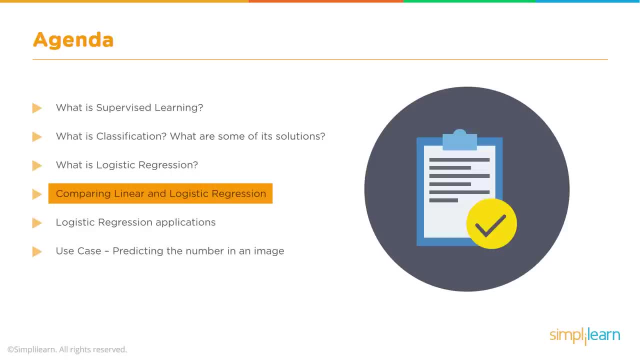 classification. Then we will compare linear and logistic regression and what are some of the logistic regression applications, And finally we will end with a use case or a demo of actual Python code for doing logistic regression in Jupyter Notebook. All right, so let's start with. 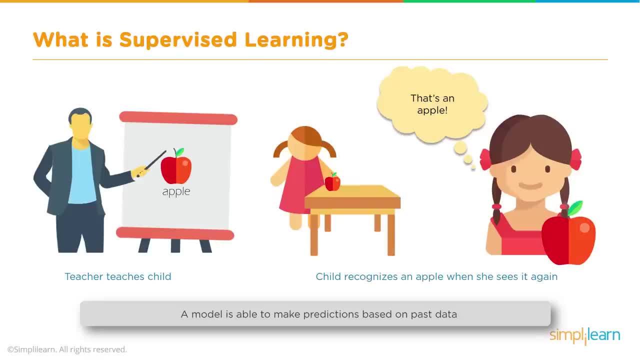 what is supervised learning? Supervised learning is one of the two main types of machine learning methods. Here we use what is known as labeled data to help the system learn. This is very similar to how we human beings learn. So let's say, you want to teach a child to recognize an apple. 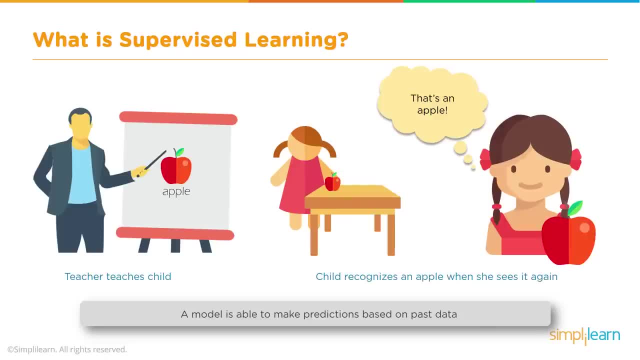 How do we do that? We never tell the child: OK, this is an apple has a certain diameter on the top, certain diameter at the bottom, this has a certain RGB color. No, we just show an apple to the child and tell the child: this is an apple. 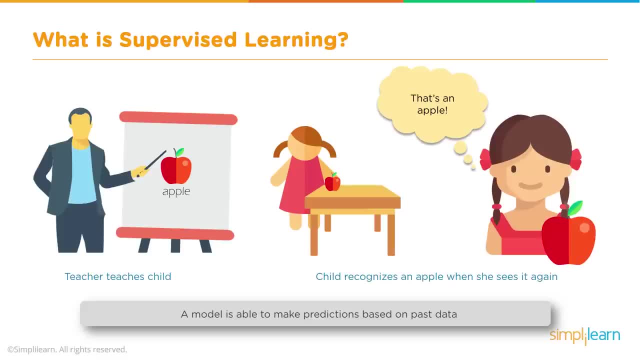 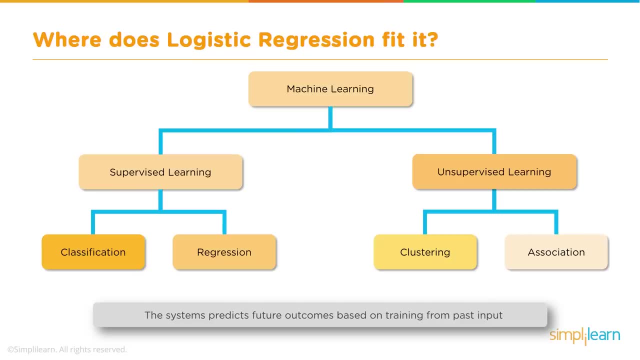 And then next time when we show an apple, child immediately recognizes: yes, this is an apple. Supervised learning works very similar on the similar lines. So where does logistic regression fit into the overall machine learning process? Machine learning is divided into two types, mainly two types. 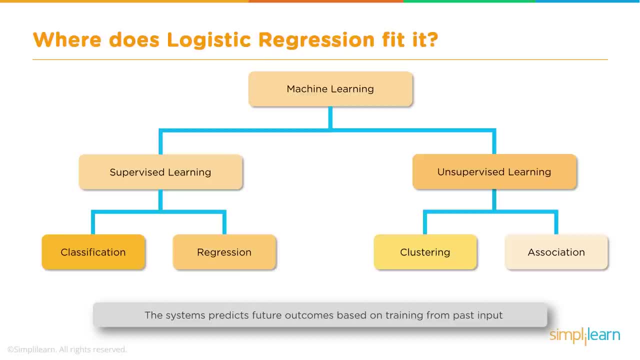 There is a third one called reinforcement learning, but we will not talk about that right now. So one is supervised learning and the other is unsupervised learning. Supervised learning uses techniques like clustering and association, and supervised learning uses techniques like classification and regression. 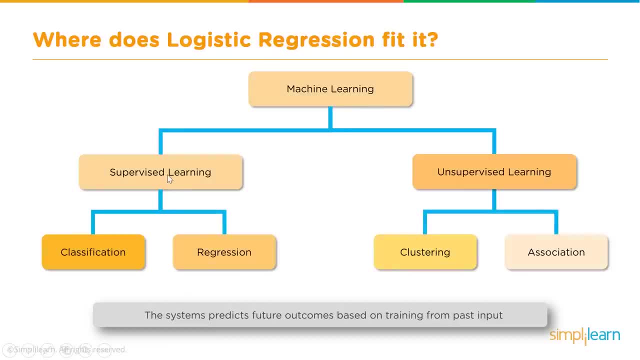 Now, supervised learning is used. when you have labeled data- you have historical data- then you use supervised learning. When you don't have labeled data, then you used unsupervised learning. In supervised learning, there are two types of techniques that are used: classification. 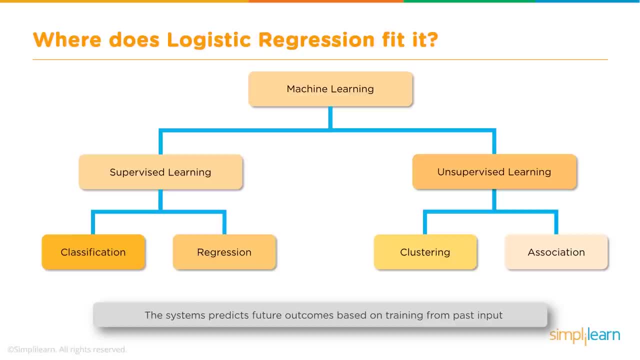 and regression based on what is the kind of problem we are solving. Let's say we want to take a problem, We take the data and classify it. It could be binary classification like a zero or a one. An example of classification: we have just seen whether the passenger has survived or 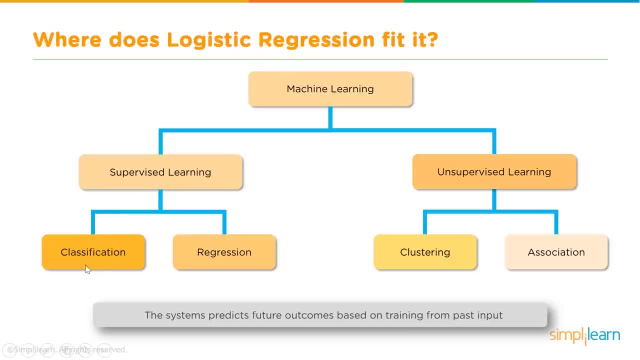 not survived. It's like a zero or one. That is known as binary classification. Regression, on the other hand, is you need to predict a value, what is known as a continuous value. Classification is for discrete values, Regression is for continuous values. 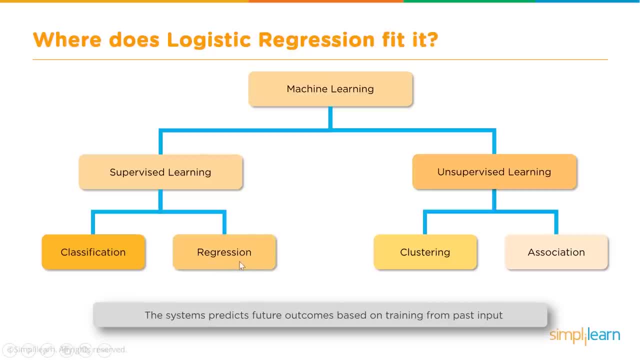 Let's say you want to predict a share price or you want to predict the temperature. What will be the temperature tomorrow? That is where you use regression, whereas classification are discrete values. Will the customer buy the product or will not buy the product? 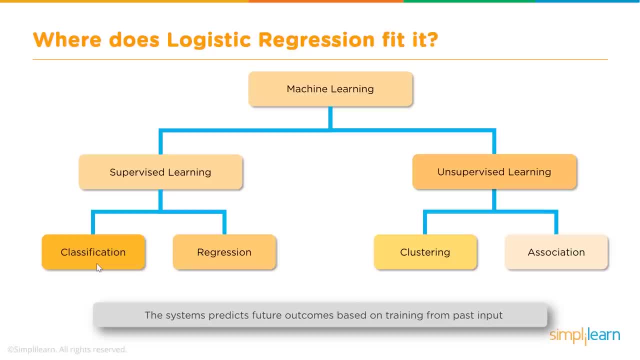 Will you get a promotion or you will not get a promotion? I hope you're getting the idea. Or it could be multi-class classification as well. Let's say you want to build an image classification model. The image classification model would take an image as an input and classify into multiple. 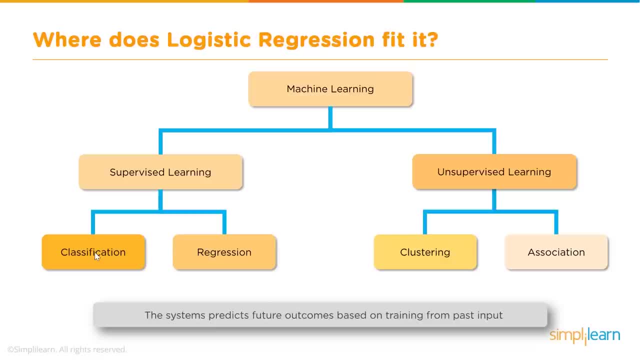 classes, whether this image is of a cat or a dog or an elephant or a tiger. So there are multiple classes, so not necessarily binary classification, So that is known as multi-class classification. So we are going to focus on classification, because logistic regression is one of the 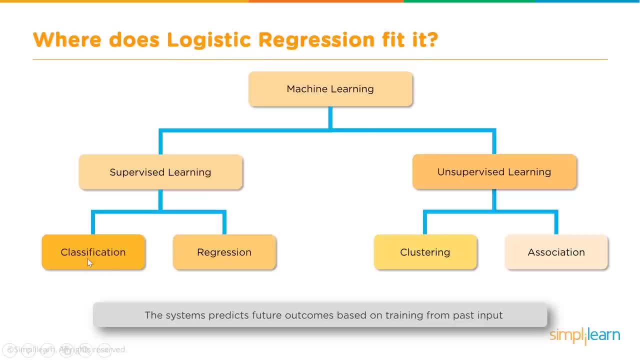 algorithms used for classification. Now, the name may be a little confusing. In fact, whenever people come across logistic regression, it always causes confusion because the name has regression in it, but we are actually using this for performing classification. So, yes, it is logistic regression, but it is used for classification. 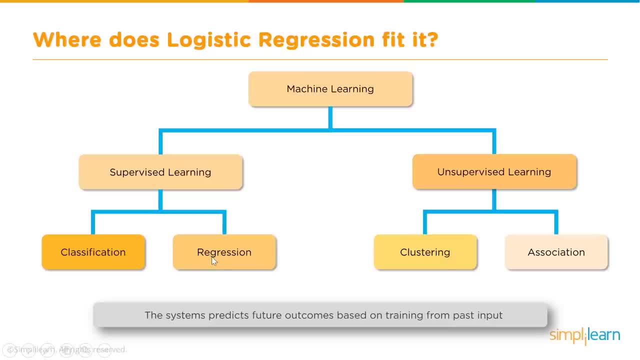 And, in case you're wondering, is there something similar for regression? Yes, For regression we have linear regression. Keep that in mind. So linear regression is used for regression. Logistic regression is used for classification. So in this video we are going to focus on supervised learning. 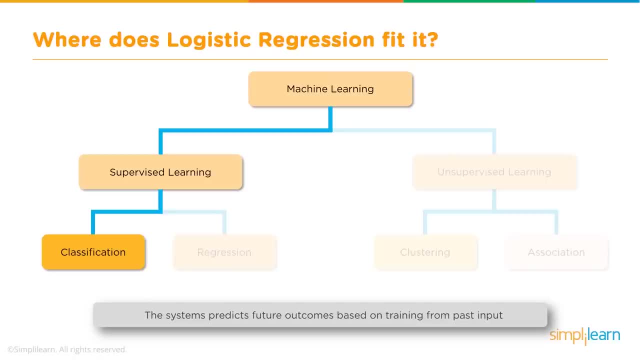 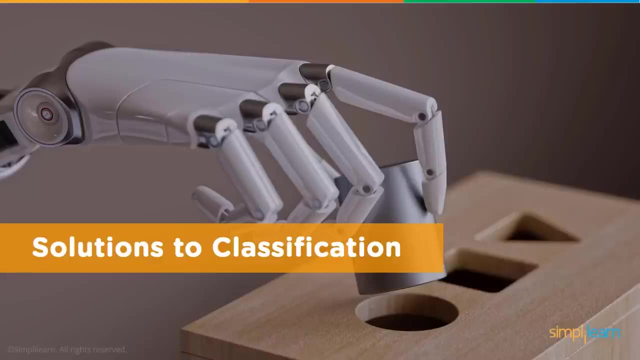 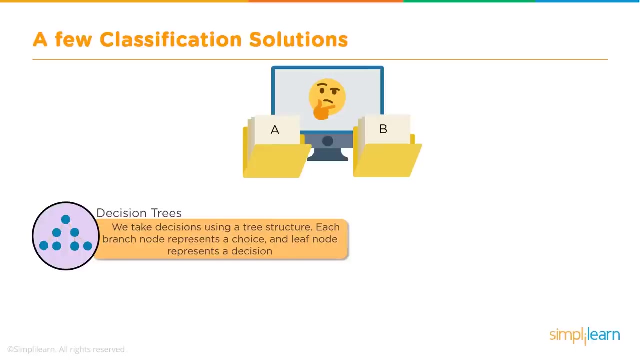 And within supervised learning, we are going to focus on classification And then, within classification, we are going to focus on logistic regression algorithm. So, first of all, classification. So what are the various algorithms available for performing classification? The first one is decision tree. 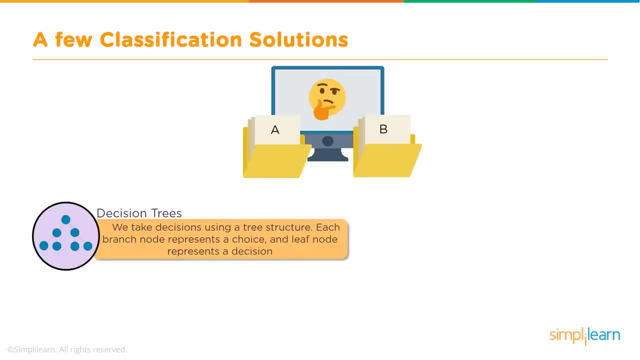 There are, of course, multiple algorithms, but here we will talk about a few. Decision trees are quite popular and very easy to understand, and therefore they're used for classification. Then we have k-nearest neighbors. This is another algorithm for performing classification. 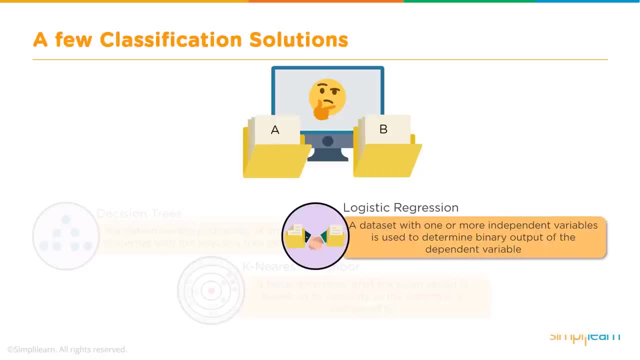 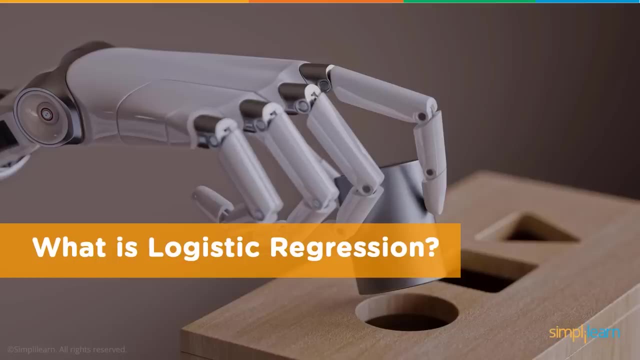 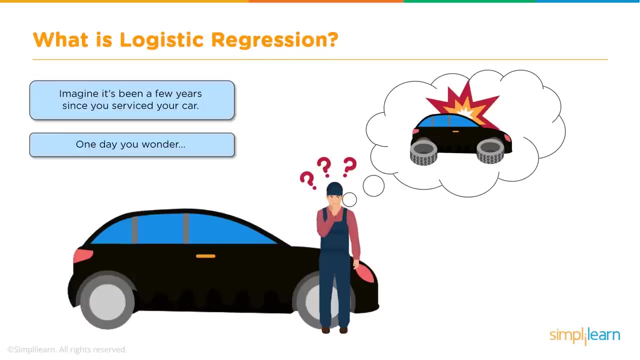 And then there is logistic regression, and this is what we are going to focus on in this video, And we are going to go into a little bit of details about logistic regression. All right, What is logistic regression? As I mentioned earlier, logistic regression is an algorithm for performing binary classification. 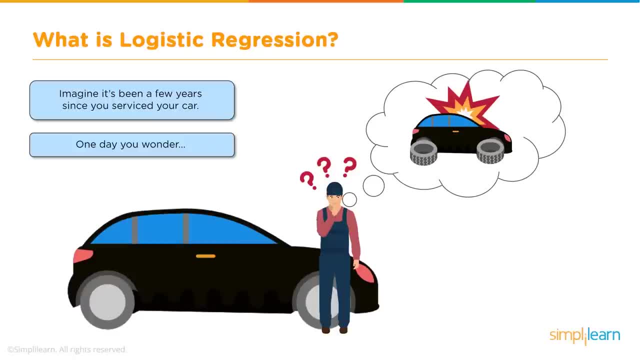 So let's take an example and see how this works. Let's say your car has not been serviced for quite a few years And now you want to find out if it is going to break down in the near future. So this is like a classification problem. 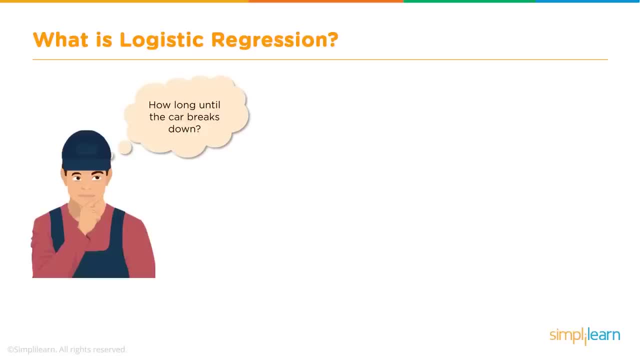 Find out whether your car will break down or not. So how are we going to perform this classification? So here's how it looks: If we plot the information along the x- and y-axis, x is the number of years since the last service was performed and y is the probability of your car breaking down. and let's say this: 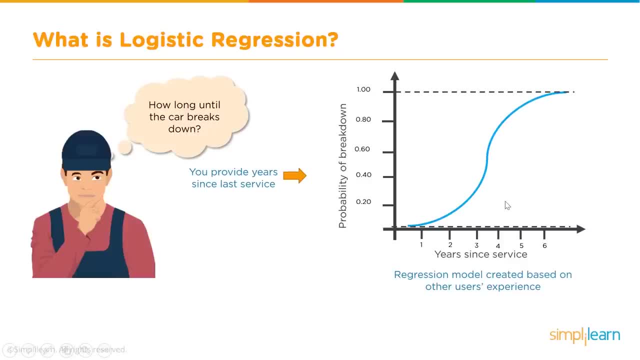 information was this: this data, rather, was collected from several car users. it's not just your car, but several car users. so that is our labeled data. so the data has been collected and for for the number of years and when the car broke down and what was the probability, and that has been plotted along. 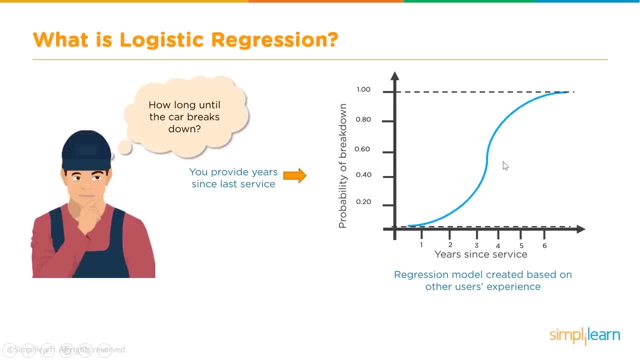 x and y axis. so this provides an idea. from this graph we can find out whether your car will break down or not. we'll see how. so, first of all, the probability can go from zero to one. as you're aware, probability can be between zero and one and, as we can imagine, it is intuitive as well. 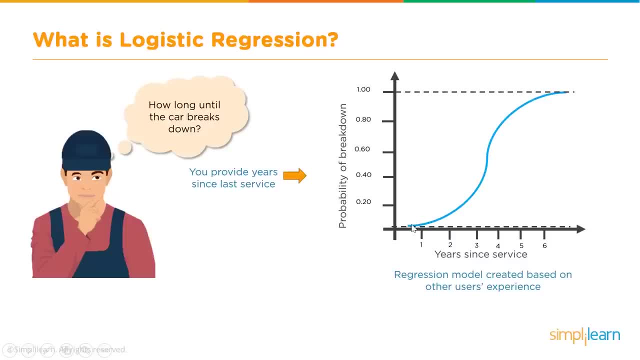 as the number of years are on the lower side- maybe one year, two years or three years till after the service- the chances of your car breaking down are very limited, right? so, for example, chances of your car breaking down or the probability of your car breaking down is very limited. 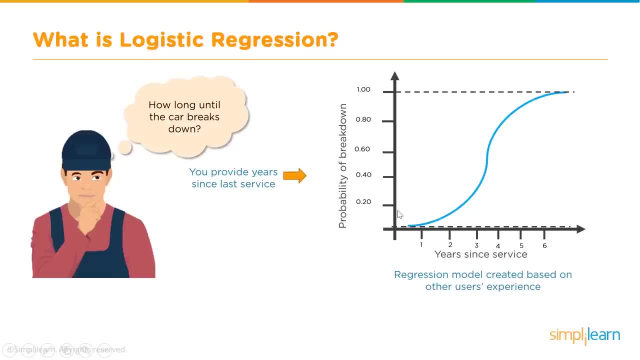 down within two years of your last service are 0.1. similarly, three years is maybe 0.3 and so on. but as the number of years increases- let's say if it was six or seven years- there is almost a certainty that your car is going to break down. that is what this graph shows. so this is an example of 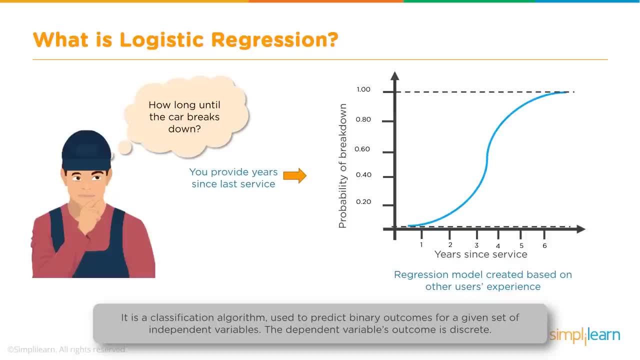 a application of the classification algorithm and we will see in little details how exactly logistic regression is applied here. one more thing needs to be added here is that the dependent variables outcome is discrete. so if we are talking about whether the car is going to break down or not, so that is a discrete value, the y that we are talking about. 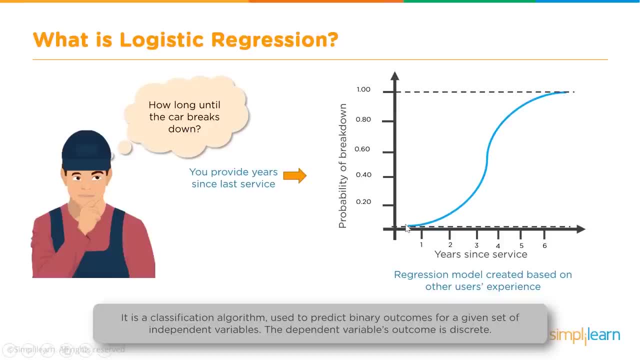 the dependent variable that we are talking about. what we are looking at is whether the car is going to break down or not, yes or no. that is what we are talking about. so here the outcome is discrete and not a continuous value. so this is how the logistic regression curve looks. let's 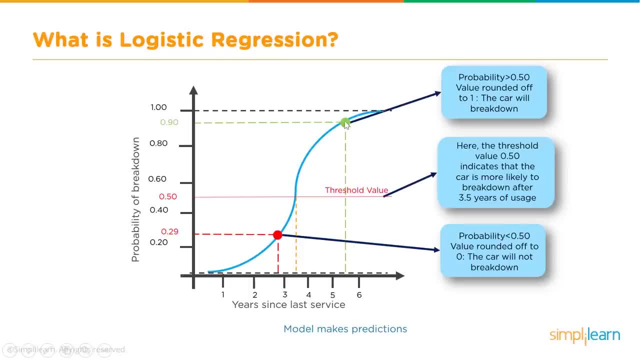 explain a little bit what exactly, how exactly we are going to determine the class at the outcome. rather so, for a logistic regression curve, a threshold has to be set. saying that, because this is a probability calculation- remember, this is a probability calculation- and the probability itself will not be 0 or 1, but based on the probability we need to decide what the outcome. 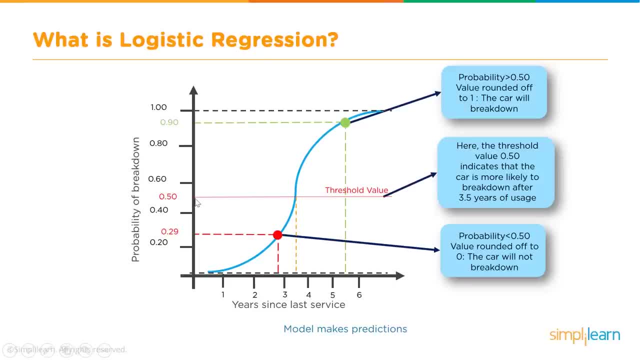 should be. so there has to be a threshold, like, for example, 0.5 can be the threshold, let's say in this case: so any value of the probability below 0.5 is considered to be 0 and any value above 0.5 is considered to be 1.. so an output of, let's say, 0.8. 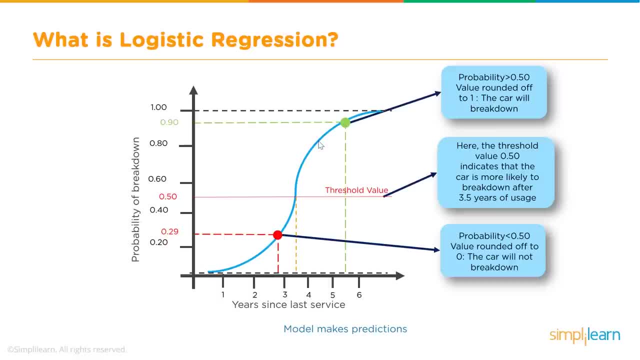 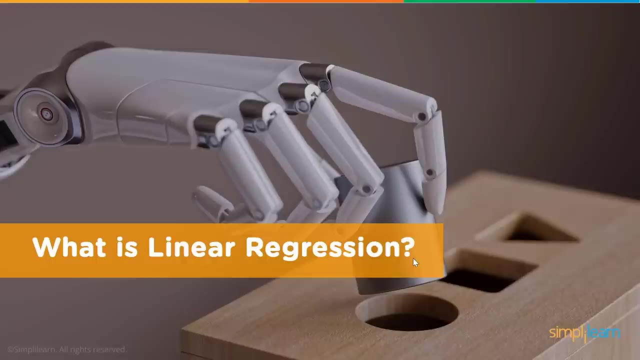 will mean that the car will break down. so that is considered as an output of 1, and let's say, an output of 0.29 is considered as 0, which means that the car will not break down. so that's the way regression works. now let's do a quick comparison between logistic regression and linear regression. 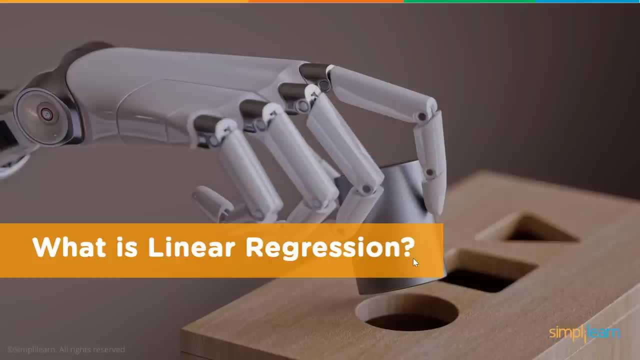 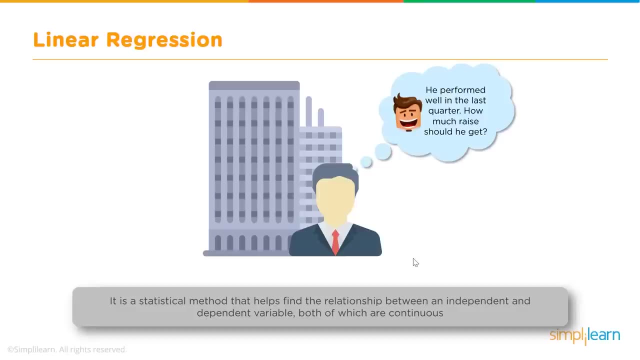 because they both have the term regression in them, so it can cause confusion. so let's try to remove that confusion. so what is linear regression? linear regression is a process, is, once again, an algorithm for supervised learning. however, here you're going to find a continuous value. you're 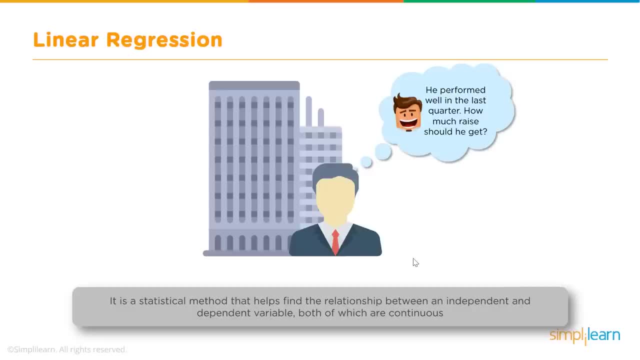 going to determine a continuous value. it could be the price of a real estate property, could be your hike, how much height you're going to get, or it could be a stock price. these are all continuous values. these are not discrete compared to a yes or no kind of response. that 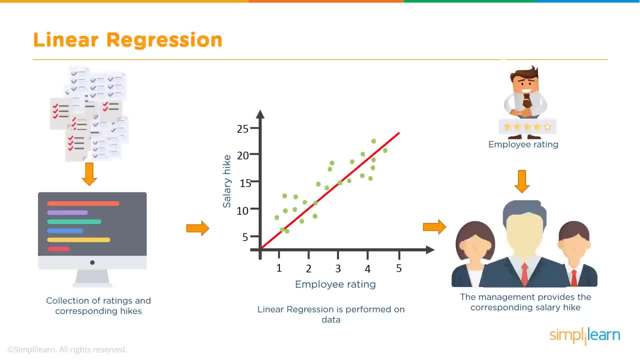 we are looking for in logistic regression. so this is one example of a linear regression. let's say the hr team of a company tries to find out what should be the salary hike of an employee, so they collect all the details of their existing employees, their ratings and their salary. 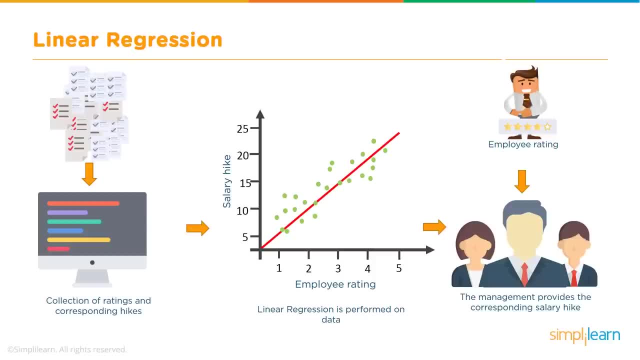 hikes what has been given and that is the labeled information that is available and the system learns from this. it is trained and it learns from this labeled information so that when a new employee's information is fed, based on the rating, it will determine what should be the height. so this is a linear regression problem and a linear 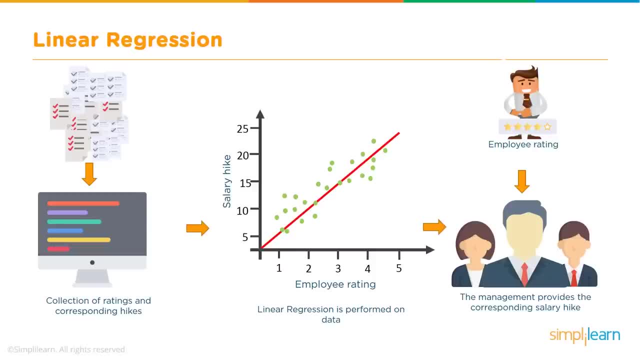 regression example. now, salary is a continuous value. you can get five thousand, five thousand, five hundred, five thousand, six hundred. it is not discrete, like a cat or a dog, apple or a banana. these are discrete, or a yes or a no. these are discrete values, right? so this? 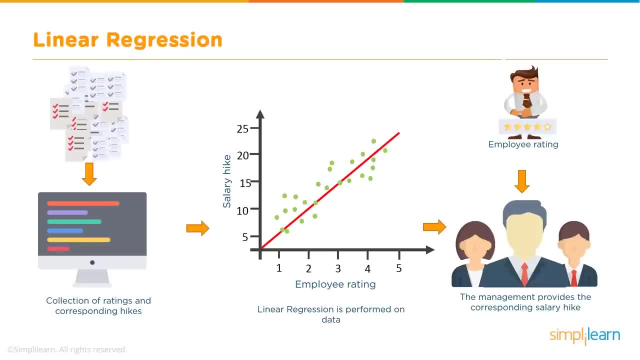 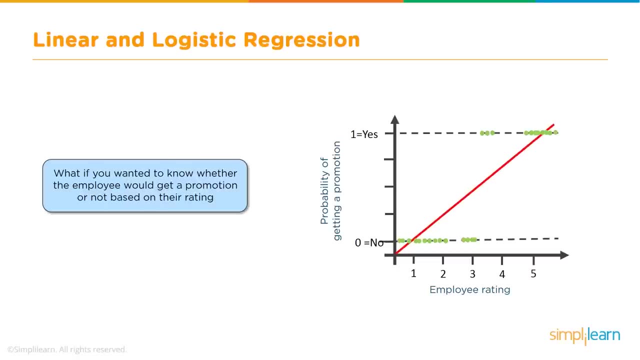 where you are trying to find continuous values is where we use linear regression. so let's say, just to extend on this scenario, we now want to find out whether this employee is going to get a promotion or not. so we want to find out. that is a discrete problem, right? a yes or no, kind of a. 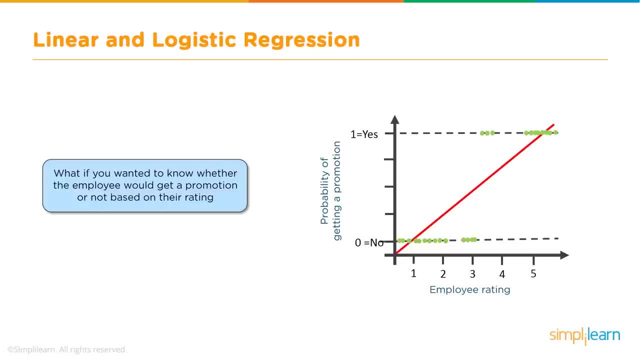 problem in this case. we actually cannot use linear regression, even though we may have labeled data. so this is the labeled data. so, based on the employee rating, these are the ratings. and then some people got the promotion and this is the ratings for which people did not get promotion. that is a no, and this is the rating for which. 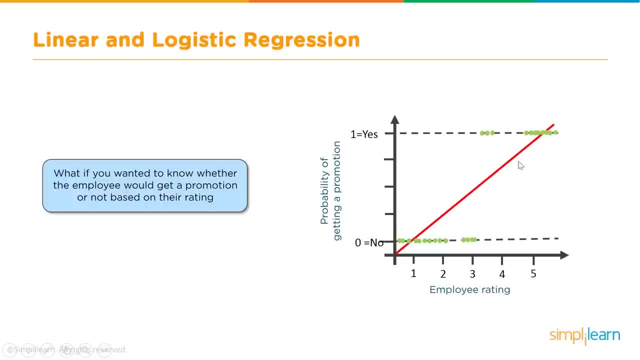 people got promotion. we just plotted the data about whether a person has got an employee has got promotion or not. yes, no, right, so there is nothing in between. and what is the employee's rating? okay, and rating is the number of employees that got promotion or not. so this is the rating. 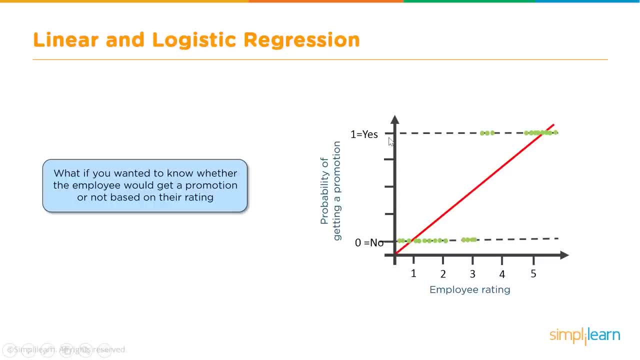 so the ratings can be continuous, that is not an issue, but the output is discrete, in this case, whether employee got promotion, yes, no, okay. so if we try to plot that and we try to find a straight line, this is how it would look and, as you can see, it doesn't look very right because, 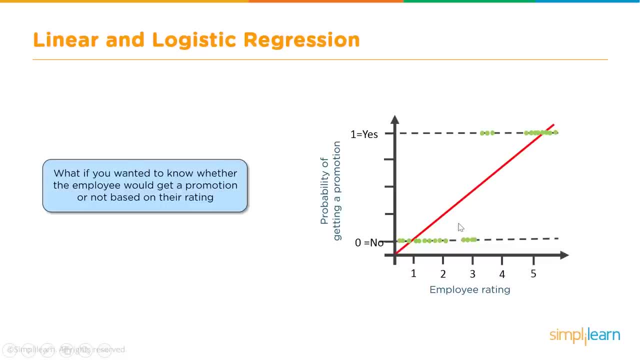 looks like there will be a lot of errors. this root mean square error, if you remember, for linear regression would be very, very high, and also the. the values cannot go beyond zero or beyond one, so graph should probably look somewhat like this: clipped at zero and one, but still the straight. 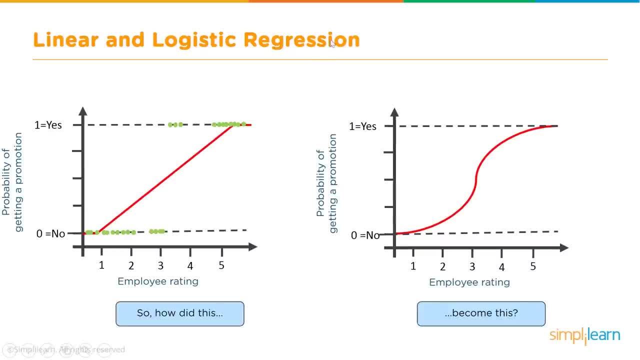 line doesn't look right. therefore, instead of using a linear equation, we need to come up with something different, and therefore the logistic regression model looks somewhat like this. so we calculate the probability and if we plot that probability- not in the form of a straight line, but we need to use some other equation. we will see very soon what that equation is. 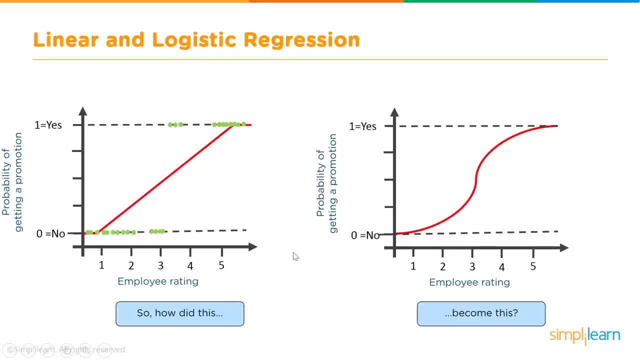 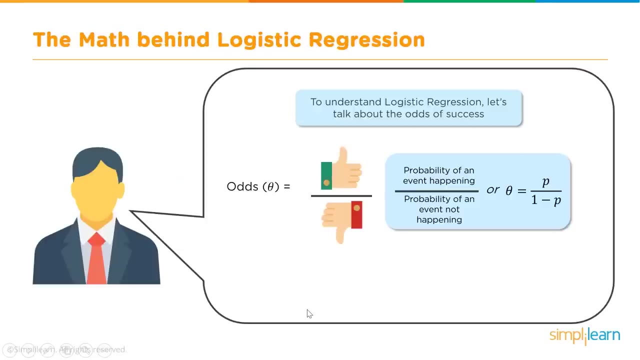 then it is a gradual process, right? so you see here, people with some of these ratings are not getting any promotions and then, slowly, at certain rating, they get promotion. so that is a gradual process and this is how the math behind logistic regression looks. so we are trying to find the odds for a. 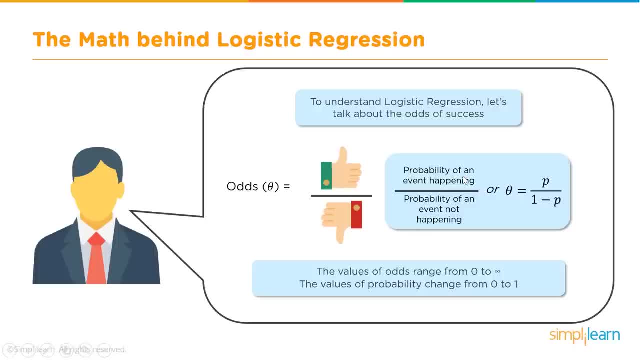 particular event happening and this is the formula for finding the odds. so the probability of an event happening divided by the probability of the event happening and then the probability of the probability of the event not happening. so p if it is the probability of the event happening- probability of the person getting a promotion- and divided by the probability of the person not. 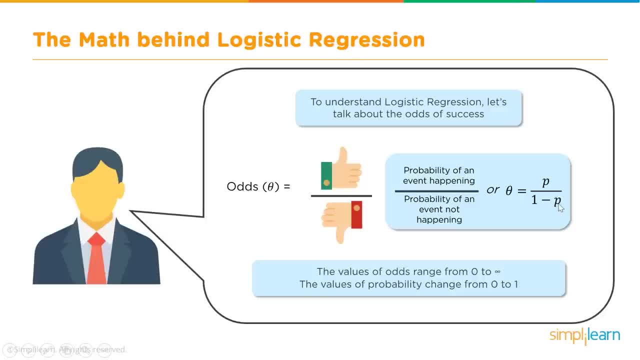 getting a promotion. that is 1 minus p. so this is how you measure the odds. now, the values of the odds range from 0 to infinity. so when this probability is 0, then the odds will. the value of the odds is equal to 0, and when the probability becomes 0, then the probability of the odds becomes. 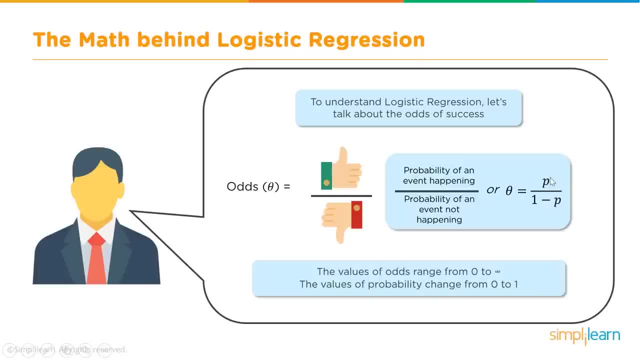 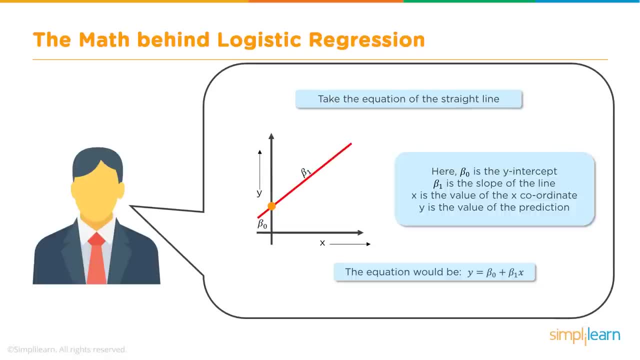 1, then the value of the odds is 1 by 0. that will be infinity, but the probability itself remains between 0 and 1.. now this is how an equation of a straight line looks. so y is equal to beta 0 plus beta 1 x, where beta 0 is a y intercept and beta 1 is the slope of the line. if we take the odds, 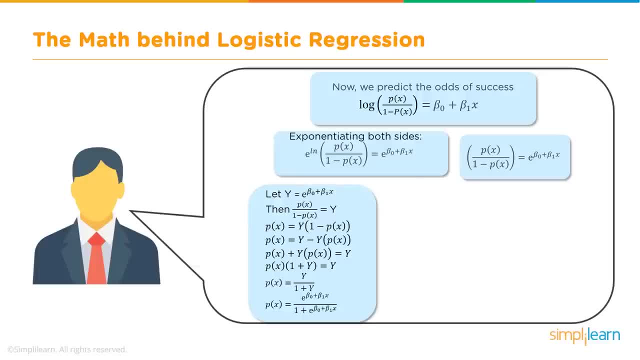 equation and take a log of both sides, then this would look somewhat like this and the term logistic is actually directly related to the log of the line, but that is also not as accurate as the from the fact that we are doing this we take a log of px by 1 minus px. this is an extension of 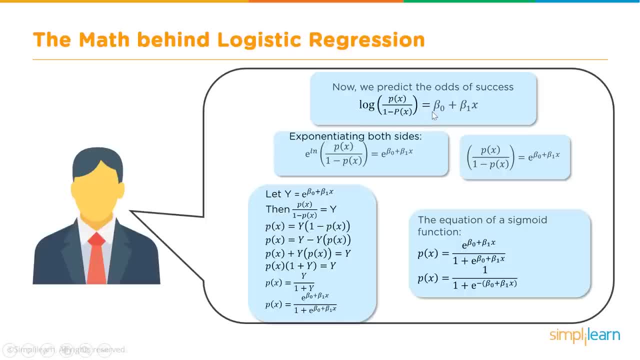 the calculation of odds that we have seen right, and that is equal to beta 0 plus beta 1x, which is the equation of the straight line. and now from here, if you want to find out the value of px, you will see we can take the exponential on both sides and then, if we solve that equation, we will get the. 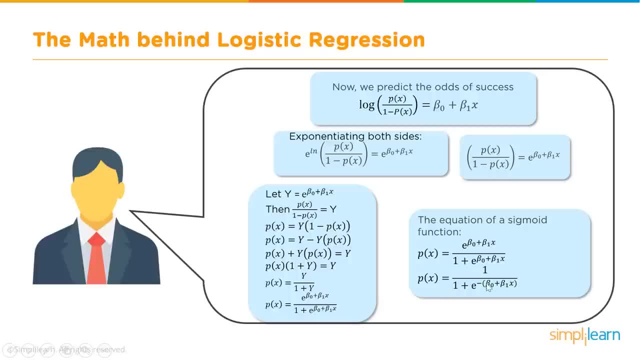 equation of px like this: px is equal to 1 by 1 plus e, to the power of minus beta 0 plus beta 1x. and recall this is nothing but the equation of the line which is equal to y, y is equal to beta 0 plus. 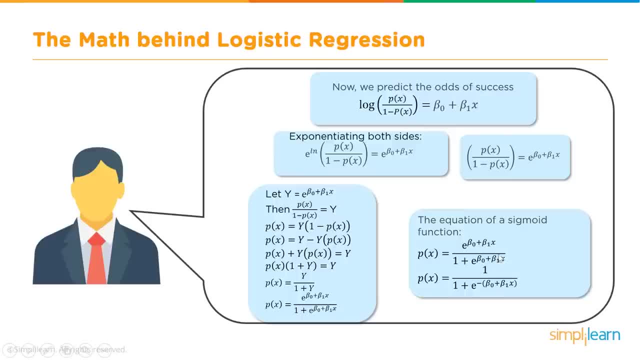 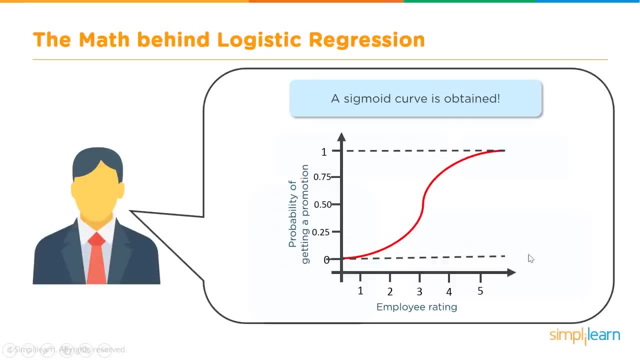 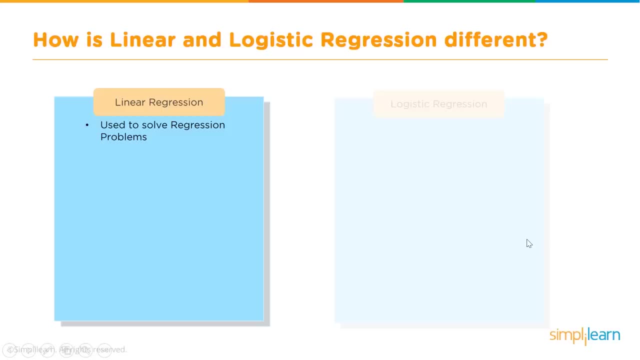 beta 1x, so that this is the equation also known as the sigmoid function, and this is the equation of the logistic regression. all right, and if this is plotted, this is how the sigmoid curve is obtained. so let's compare linear and logistic regression how they are different from each other. let's go back, so linear. 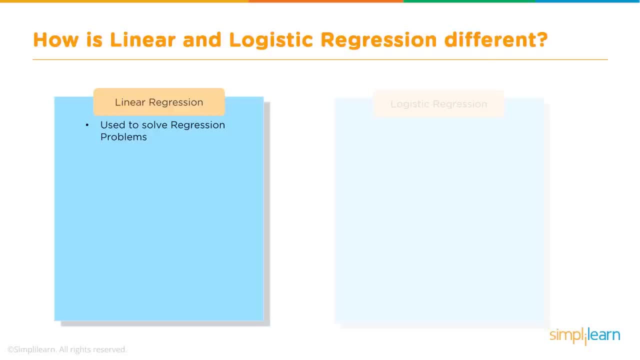 regression is solved or used to solve regression problems and logistic regression is used to solve classification problems, so both are called regression. but linear regression is used for solving regression problems where we predict continuous values, whereas logistic regression is used for solving classification problems where we have have to predict. 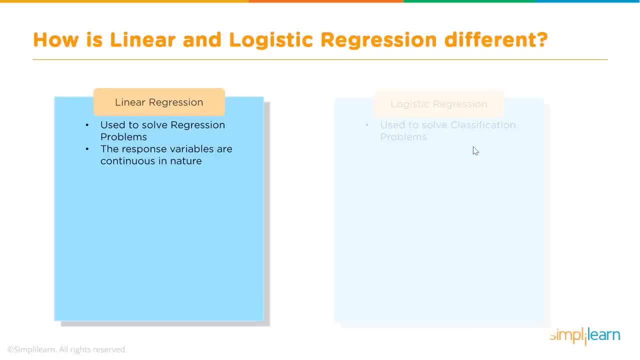 this discrete values. the response variables in case of linear regression are continuous in nature, whereas here they are categorical or discrete in nature. and linear regression helps to estimate the dependent variable when there is a change in the independent variable, whereas here, in case of logistic regression, it helps to calculate the probability or the possibility of a particular. 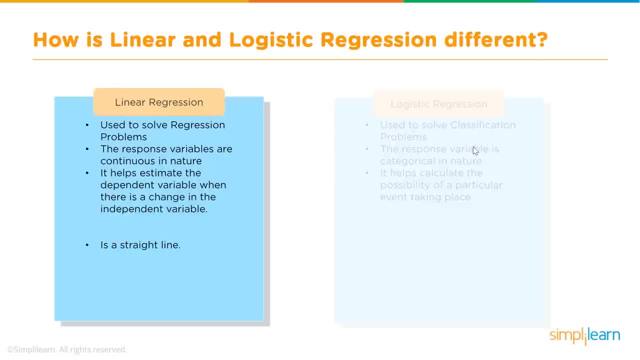 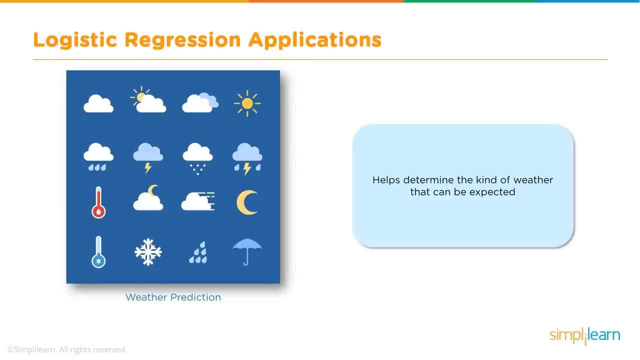 event happening and linear regression, as the name suggests, is a straight line. that's why it's called linear regression, whereas logistic regression is a sigmoid function and the curve is. the shape of the curve is s, it's an S-shaped curve. this is another example of application of logistic regression in weather. 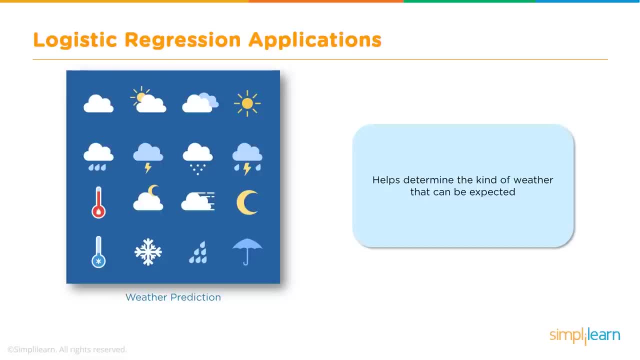 prediction whether it's going to rain or not rain. now, keep in mind both are used in weather prediction. if we want to find the discrete values, like whether it's going to rain or not rain- that is a classification problem- we use logistic regression. but if we want to determine what is going to rain, so logistic regression is an application or is a way for 매pective regression. case of when: 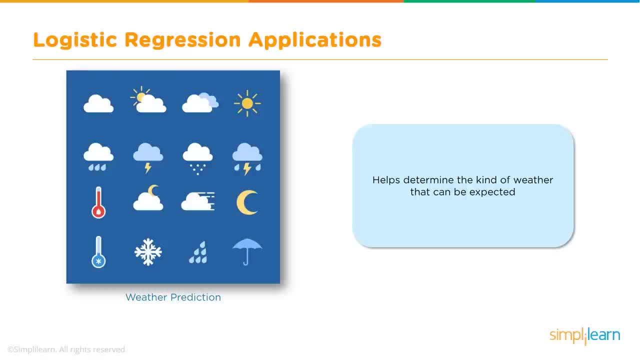 problem. We use logistic regression, But if we want to determine what is going to be the temperature tomorrow, then we use linear regression. So just keep in mind that in weather prediction we actually use both. But these are some examples of logistic regression. So we want 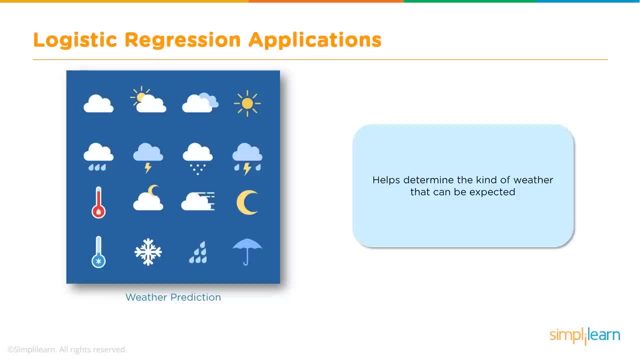 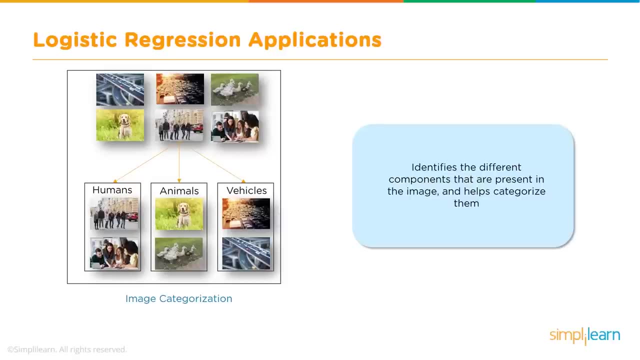 to find out whether it's going to rain or not, Is it going to be sunny or not, Is it going to snow or not. These are all logistic regression examples. A few more examples: Classification of objects. This is again another example of logistic regression. Now here, of course, one distinction. 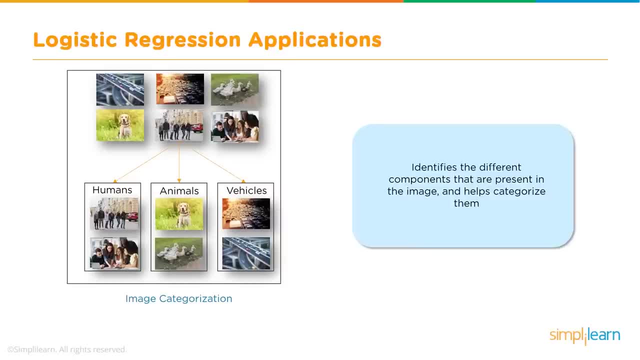 is that these are multi-class classification, So logistic regression is not used in its original form, but it is used in a slightly different form. So we say: whether it is a dog or not a dog. I hope you understand. So instead of saying: is it a dog or a cat or elephant, we convert this into saying: 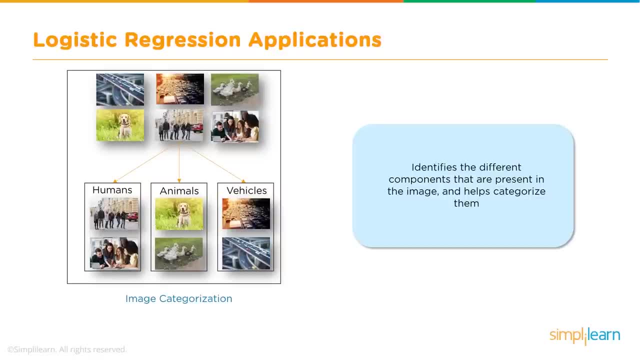 So because we need to keep it to binary classification. so we say: is it a dog or not a dog, Is it a cat or not a cat? So that's the way logistic regression can be used for classifying objects. Otherwise there are other techniques which can. 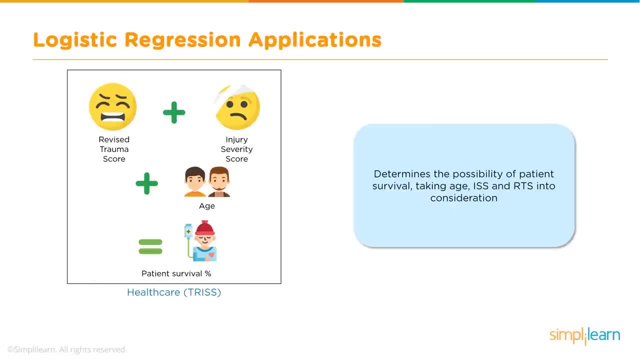 be used for performing multi-class classification In healthcare. logistic regression is used to find the survival rate of a patient, So they take multiple parameters like trauma score and age and so on and so forth, And they try to predict the rate of survival. All right. So that's the way logistic regression can be used for classifying objects. So we say: is it a dog or not a dog, Is it a cat or not a cat? So that's the way logistic regression can be used for. 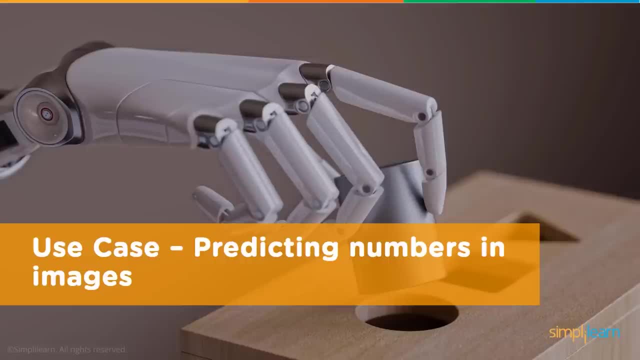 classifying objects. All right Now, finally, let's take an example and see how we can apply logistic regression to predict the number that is shown in the image. So this is actually a live demo. I will take you into Jupyter Notebook and show the code, But before that, let me take you. 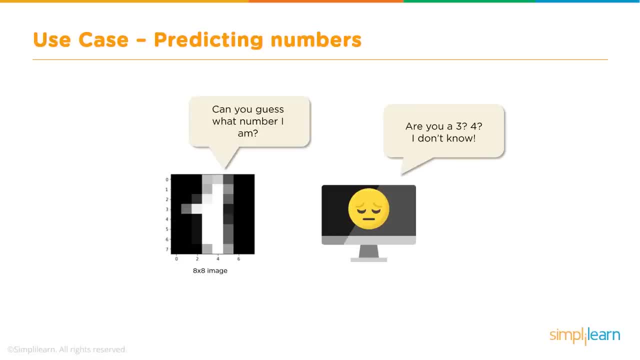 through a couple of slides to explain what we are trying to do. So let's say you have an 8x8 image and the image has a number 1,, 2,, 3,, 4.. And you need to train your model to predict what this. 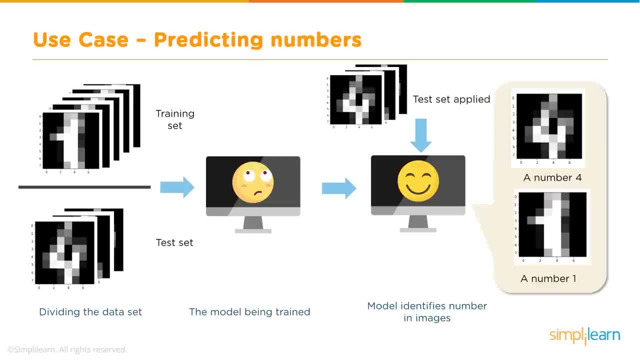 number is. So let's say, you have an 8x8 image and the image has a number: 1,, 2,, 3,, 4.. And you need to train your model to predict what this number is. So how do we do this? So the first thing is: 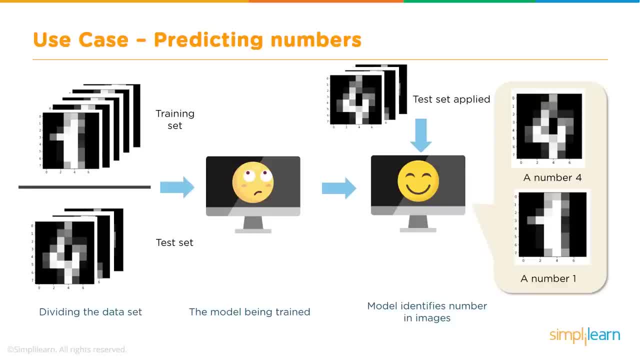 obviously, in any machine learning process, you train your model. So in this case, we are using logistic regression. So and then we provide a training set to train the model, And then we test how accurate our model is with the test data. which means that, like any machine learning process, 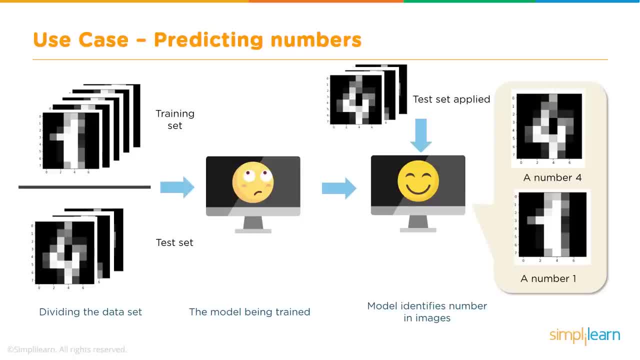 we split our initial data into two parts: training set and test set. With the training set, we train our model, And then, with the test set, we test the model And then we get good accuracy And then we use it for inference right. So that is typical. 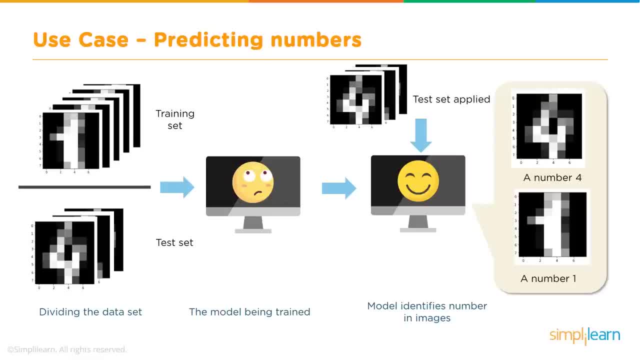 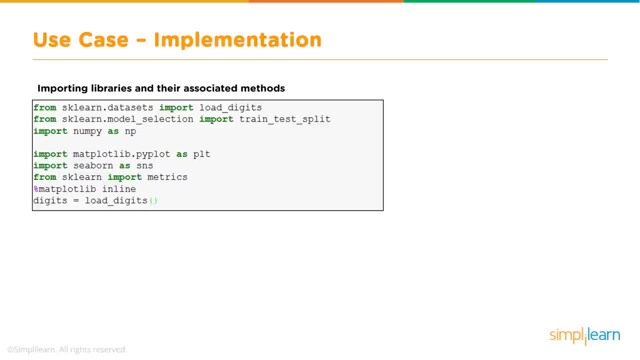 methodology of training, testing and then deploying of machine learning models. So let's take a look at the code and see what we are doing. So I will not go line by line, but just take you through some of the blocks. So first thing we do is import all the libraries And then we basically 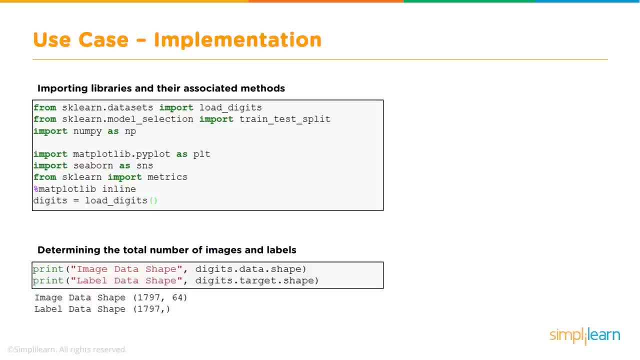 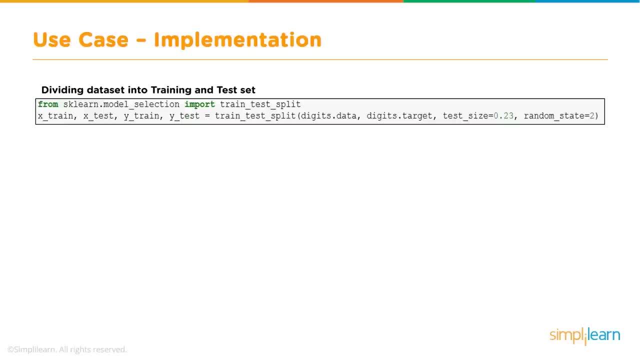 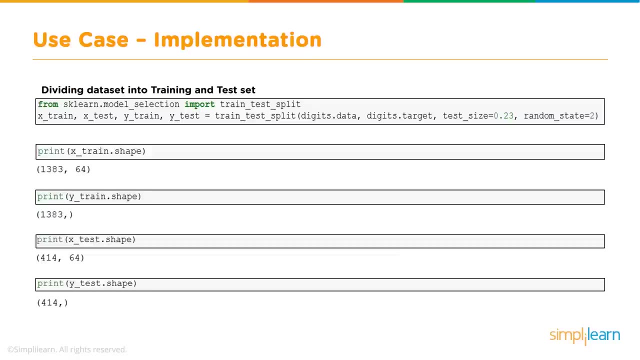 take a look at the images and see what is the total number of images. We can display using matplotlib some of the images or a sample of these images, And then we split the data into training and test, as I mentioned earlier, And we can do some exploratory analysis And then 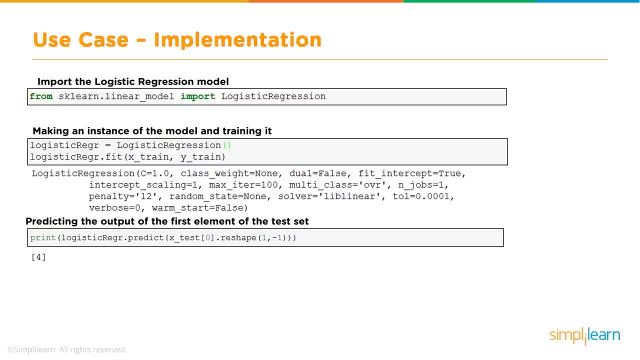 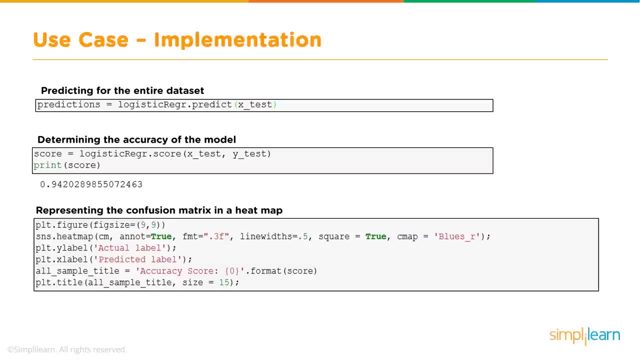 we build our model, we train our model with the training set And then we test it with our test set and find out how accurate our model is using the confusion matrix, the heat map, and use heat map for visualizing this And I will show you. 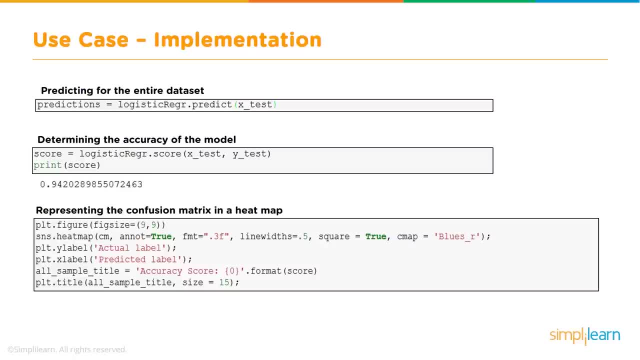 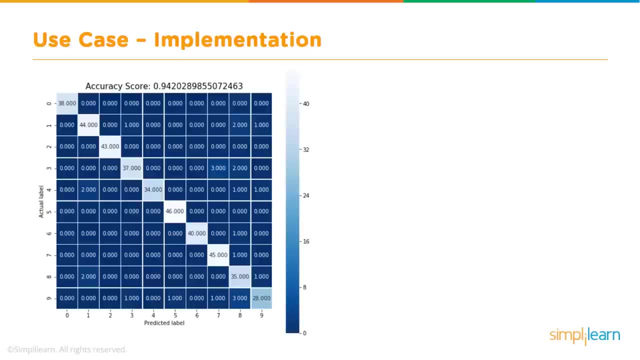 in the code, what exactly is the confusion matrix and how it can be used for finding the accuracy. In our example we got, we get an accuracy of about 0.94,, which is pretty good, or 94%, which is pretty good, All right. So what is the confusion matrix? This is an example of 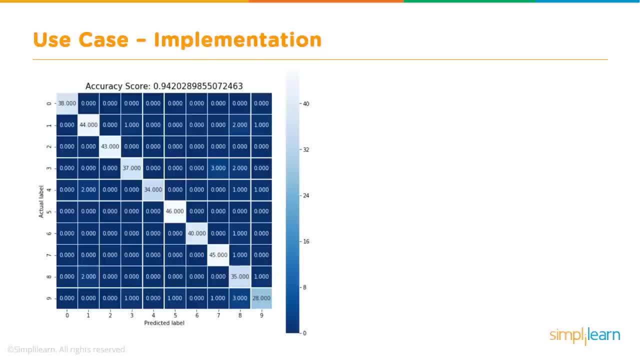 a confusion matrix And this is used for identifying the accuracy of a classification model like a logistic regression model. So the most important part in studying confsky and a confusion matrix is that, first of all, this: as you can see, this is a matrix and the size of the matrix depends on how many outputs we are expecting. 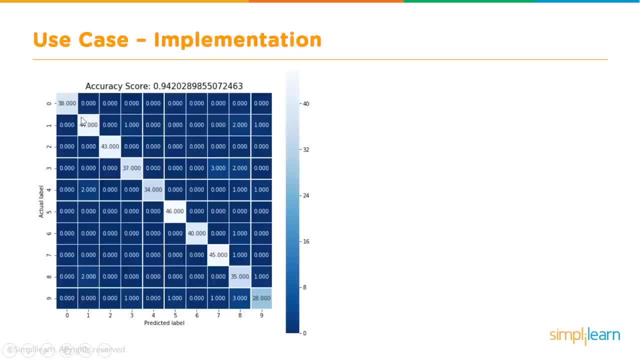 Right. So the most important part here is that the model will be most accurate when we have the maximum numbers in its diagonal, Like in this case. that site has almost 93, 94%, because the diagonal should have the maximum numbers And the others other than diagonal. these are the 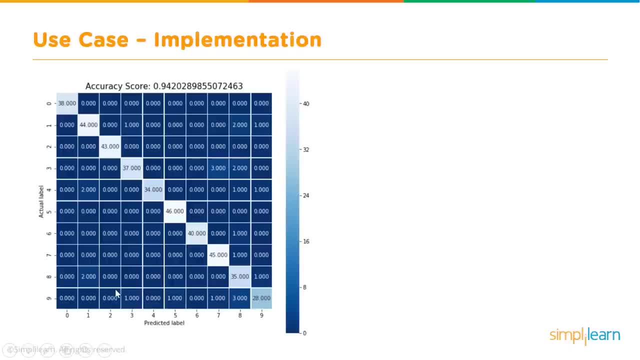 the cells other than the diagonals should have very few numbers. so here that's what is happening. so there is a two here, there are, there's a one here, but most of them are along the diagonal this. what does this mean? this means that the number that has been fed is zero and the number 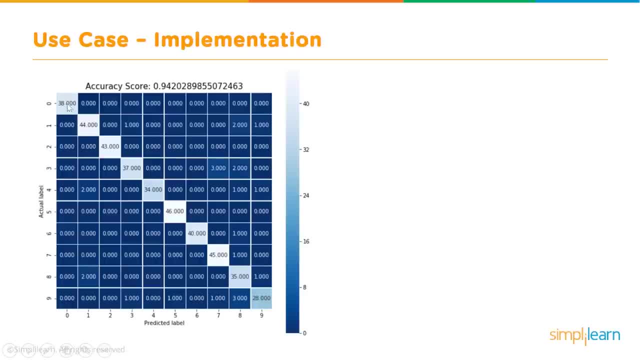 that has been detected is also zero. so the predicted value and the actual value are the same. so, along the diagonals, that is true, which means that let's, let's take this diagonal right. if the maximum number is here, that means that, like here, in this case, it is 34, which means that 34 of the 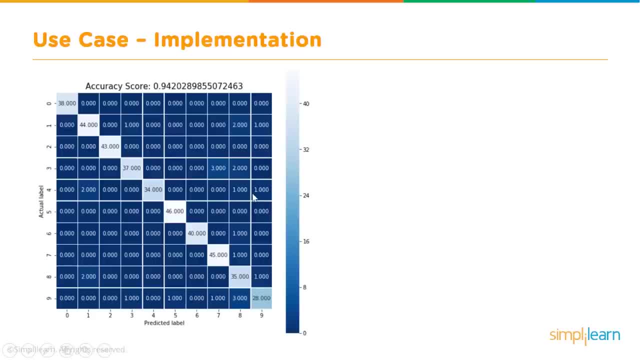 images that have been fed, or rather, actually there are two misclassifications in there. so 36 images have been fed which have number four, and out of which 34 have been predicted correctly as number four and one has been predicted as number eight and three have been predicted as number six, and so on, which are the different types of numbers. 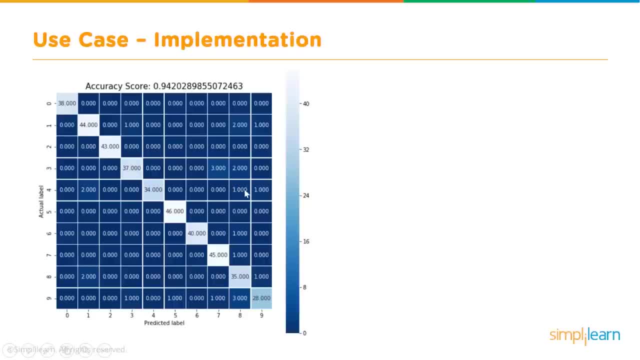 another one has been predicted as number nine, so these are two misclassifications. okay, so that is the meaning of saying that the maximum number should be in the diagonal. so if you have all of them, so for an ideal model which has, let's say, 100 accuracy, everything will be. 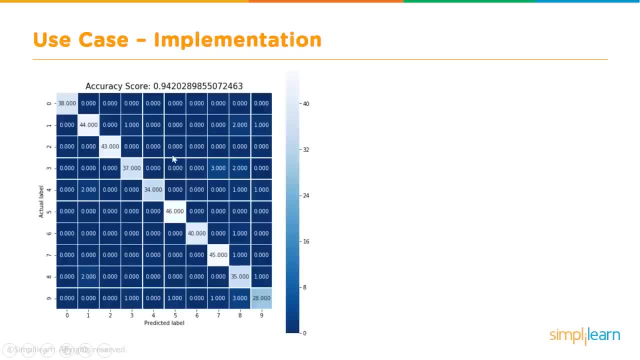 only in the diagonal. there will be no numbers other than zero in all other cells. so that is like a hundred percent accurate model. okay, so that's uh just of how to use this matrix. uh, how to use this uh confusion matrix. i know the name uh is a little funny sounding: confusion matrix. 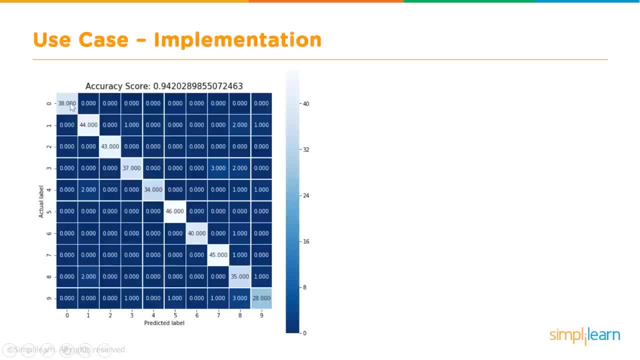 but actually it is not very confusing, it's very straightforward. so you are just plotting what has been predicted and what is the labeled information or what is the actual data. that's also known as the ground truth sometimes- okay, these are some fancy terms that are used. so: predicted label. 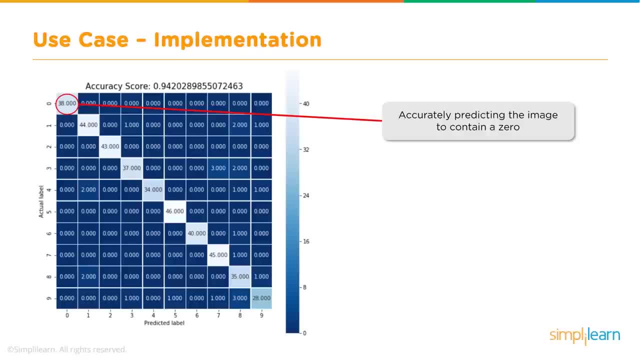 and the actual name. that's all it is okay. yeah, so we are showing a little bit more information here. so 38 have been predicted and here you will see that all of them have been predicted correctly. there have been 38 zeros and the predicted value and the actual value is exactly the same, whereas in this case, 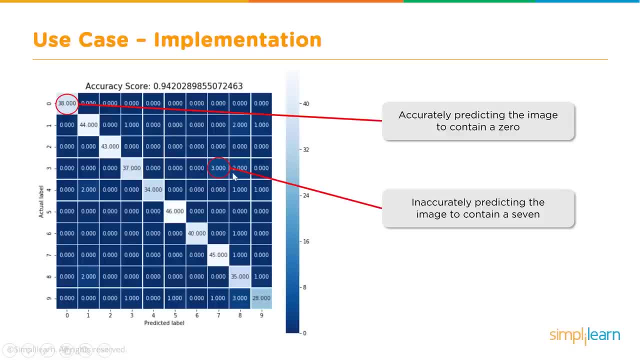 right, it has. uh, there are i think 37 plus five. yeah, 42 have been fed the images. 42 images are of digit 3 and the accuracy is only 37 of them have been accurately predict. three of them have been predicted as number seven and two. 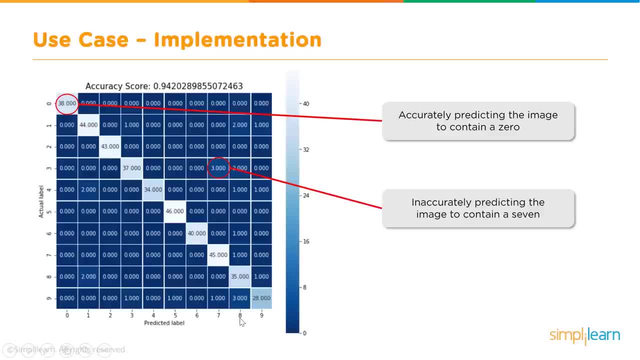 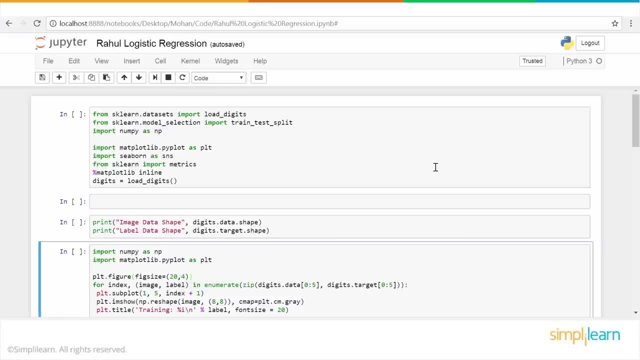 them have been predicted as number eight and so on and so forth. okay, all right. so with that, let's go into jupyter notebook and see how the code looks. so this is the code in in jupyter notebook for logistic regression. in this particular demo, what we are going to do is train our model to 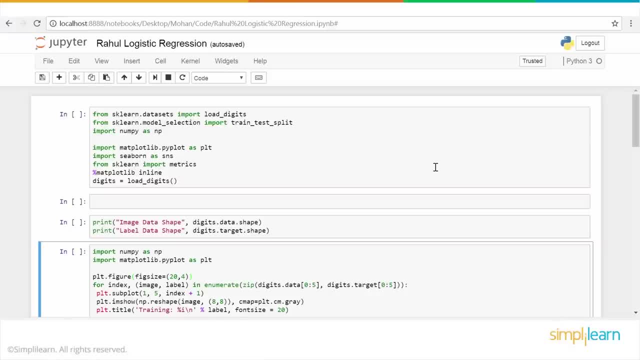 recognize digits, which are the images which have digits from, let's say, zero to five or zero to nine, and and then we will see how well it is trained and whether it is able to predict these numbers correctly or not. so let's get started. so the first part is, as usual, we are importing some libraries. 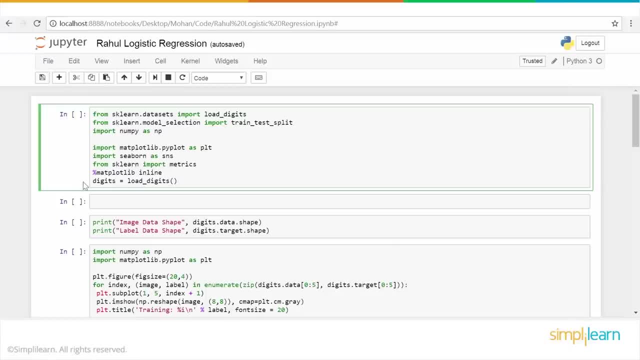 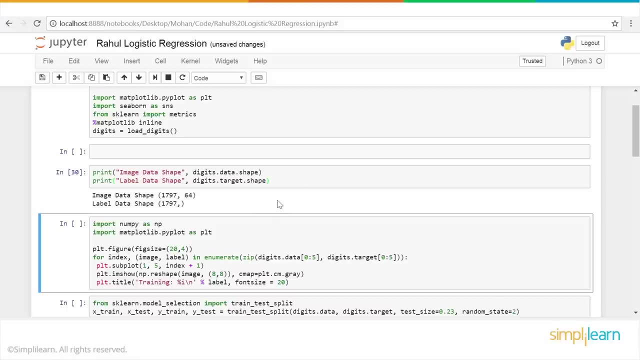 that are required. and then the last line and this block is to load the digits. so let's go ahead and run this code, then here we will visualize the shape of these digits so we can see here. if we take a look, this is how the shape is: 1797 by 64. these are like 8 by 8 images. 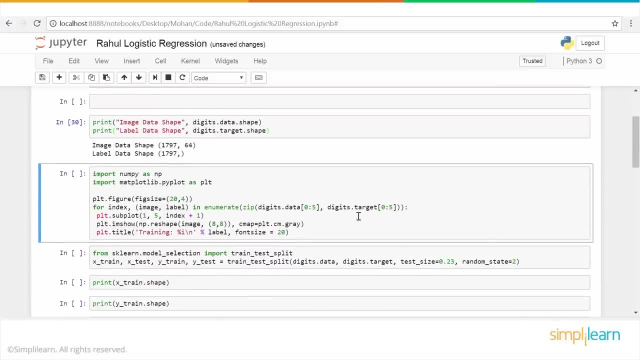 so that's, that's what is reflected in this shape. now, from here onwards, we are basically once again importing some of the libraries that are required, like numpy and matplot, and we will take a look at some of the sample images that we have loaded. so this one, for example, creates a figure and then we go ahead and take a look at the sample images that we have loaded. so this one, for example, creates a figure. and then we go ahead and take a look at the sample images that we have loaded. so this one, for example, creates a figure, and then we go ahead and take. 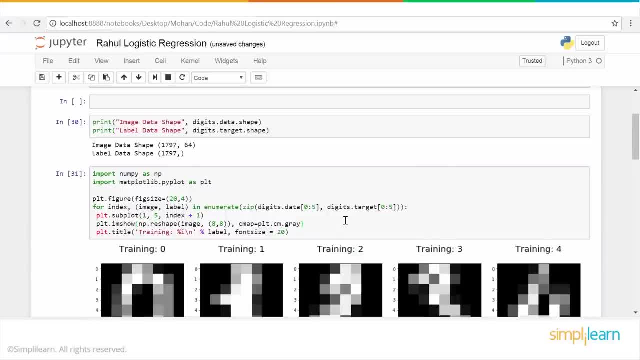 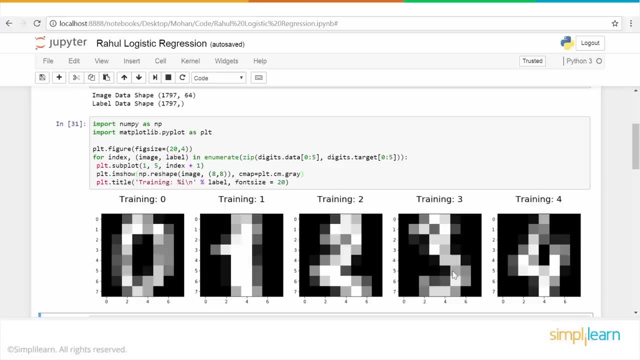 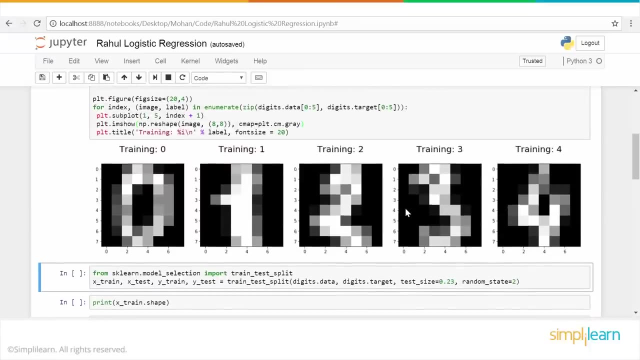 a few sample images to see how they look. so let me run this code and so that it becomes easy to understand. so these are about five images, sample images that we are looking at: zero, one, two, three, four. so this is how the images, this is how the data is okay and based on this, we will actually 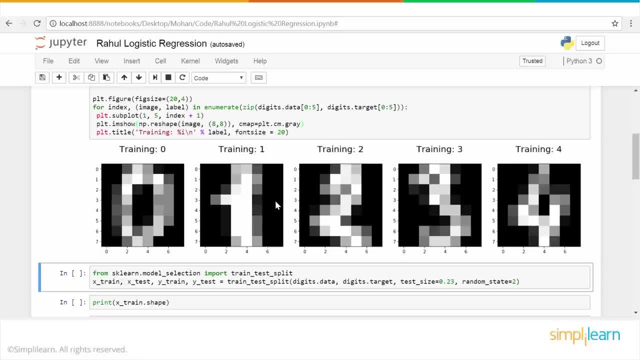 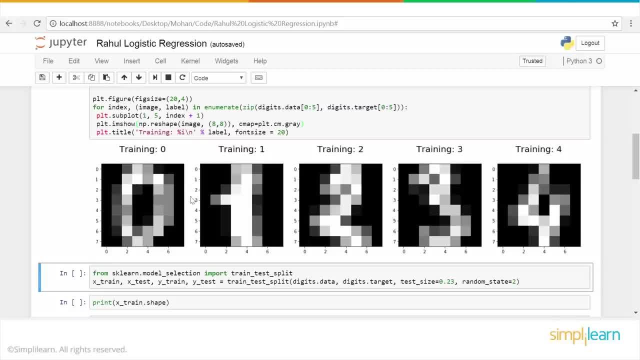 the way it works is the pixel information, so, as you can see here this pixel information, so as you can see here this pixel information, so as you can see here, this is an eight by eight pixel kind of a. is an eight by eight pixel kind of a. 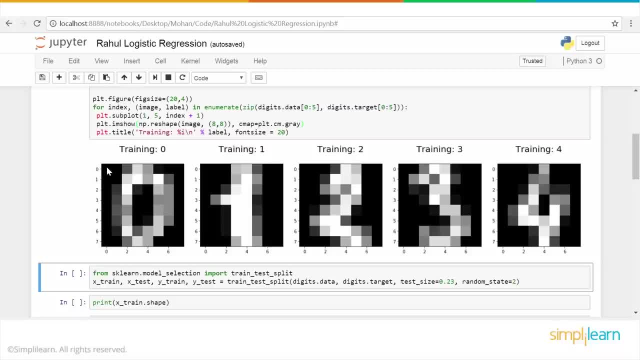 is an eight by eight pixel kind of a image and image and image and the each pixel, whether it is activated, or the each pixel, whether it is activated or the each pixel, whether it is activated or not activated, that is the information. not activated, that is the information. 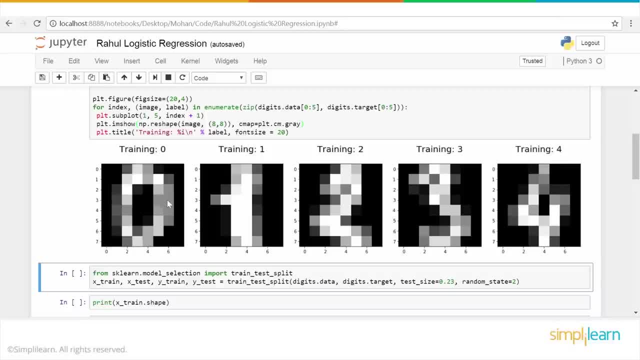 not activated. that is, the information available for each pixel now, based on the available for each pixel now. based on the available for each pixel now, based on the pattern of this activation and pattern of this activation and pattern of this activation and non-activation of the various pixels. 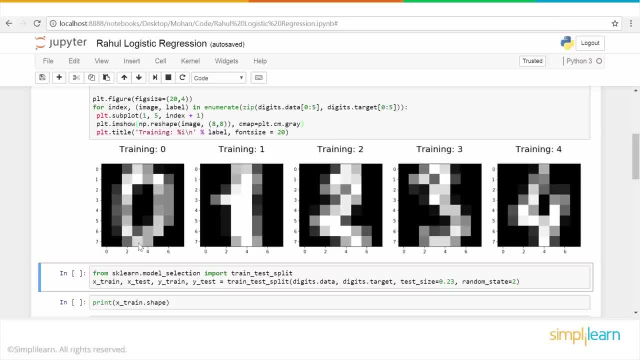 non-activation of the various pixels. non-activation of the various pixels. this will be identified as a zero. for this will be identified as a zero. for this will be identified as a zero. for example, right. similarly as you can see. example right. similarly as you can see. 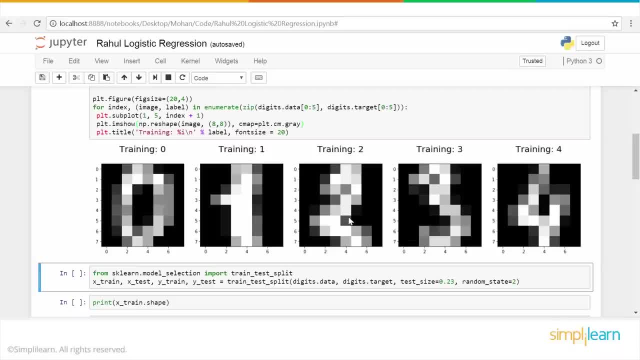 example, right, similarly, as you can see. so, overall, each of these numbers actually so overall, each of these numbers actually so overall, each of these numbers actually has a different pattern of the pixel, has a different pattern of the pixel, has a different pattern of the pixel activation, and that's pretty much that. 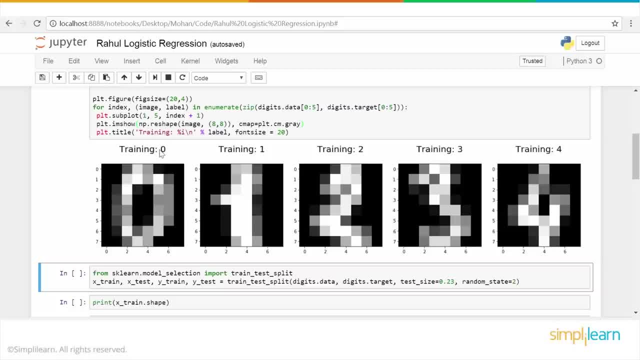 activation, and that's pretty much that activation, and that's pretty much that our model needs to learn. our model needs to learn. our model needs to learn: for which a number? what is the pattern for which a number? what is the pattern for which a number? what is the pattern of the activation of the pixels? right, so? 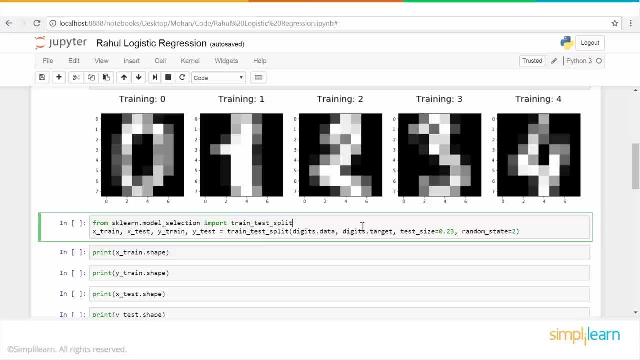 of the activation of the pixels, right. so of the activation of the pixels, right. so that is what we are going to train our, that is what we are going to train our, that is what we are going to train our model. okay, so the first thing we need to 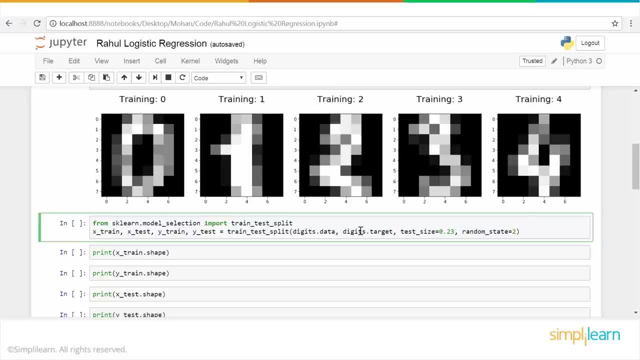 model okay. so the first thing we need to model, okay. so the first thing we need to do is to split our data into training. do is to split our data into training. do is to split our data into training and test. data set right- so whenever we- and test data set right- so whenever we. 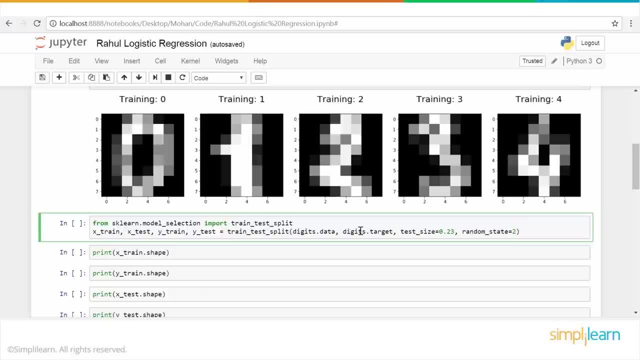 and test data set right. so whenever we perform any training, we split the data. perform any training. we split the data. perform any training. we split the data into training and test so that the into training and test, so that the into training and test, so that the training data set is used to train the. 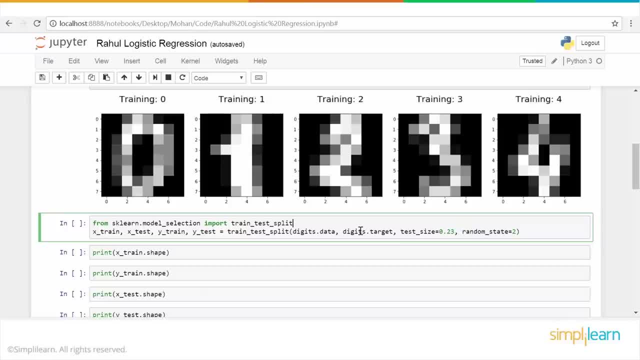 training data set is used to train the training data set is used to train the system. so we pass this probably multiple system. so we pass this probably multiple system. so we pass this probably multiple times, times times. and then we test it with the test data, and then we test it with the test data set and the split is usually in the form: 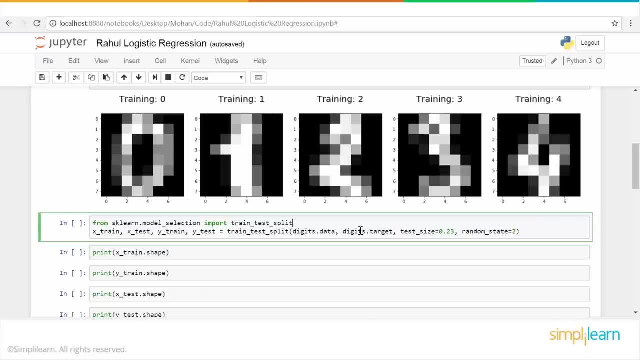 set and the split is usually in the form set and the split is usually in the form of the and there are various ways in of the and there are various ways in of the and there are various ways in which you can split this data. it is up. 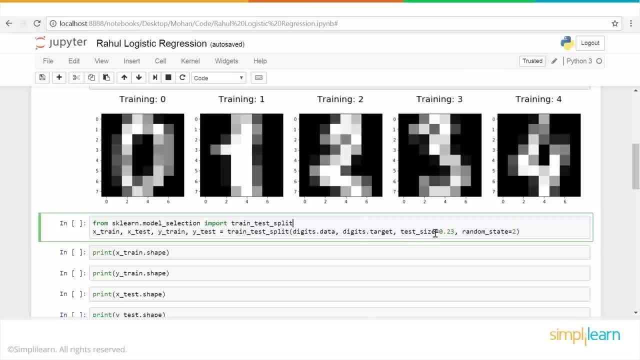 which you can split this data. it is up which you can split this data. it is up to the individual preferences in our, to the individual preferences in our, to the individual preferences in our case. here we are splitting in the form. case: here we are splitting in the form. 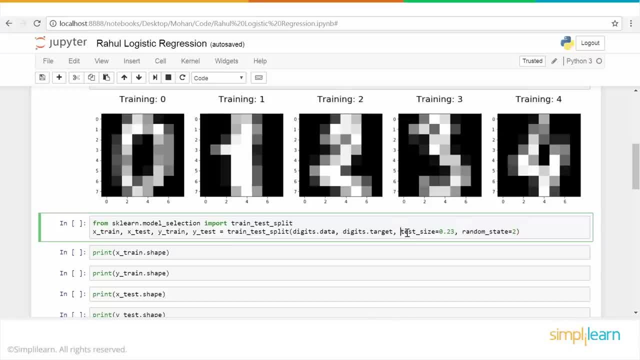 case. here we are splitting in the form of 23 and 77. so when we say test size as of 23 and 77, so when we say test size as of 23 and 77, so when we say test size as 20.23, that means 23 percent of that. 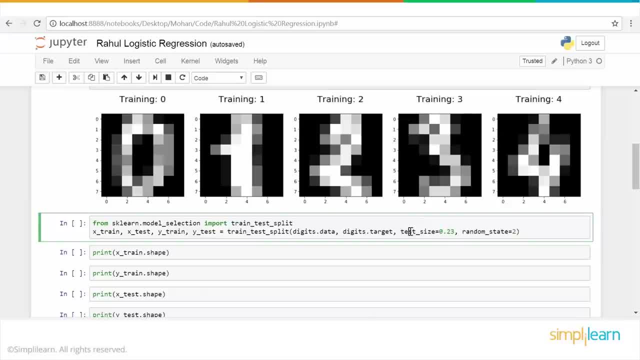 20.23. that means 23 percent of that. 20.23. that means 23 percent of that. entire data is used for testing and the entire data is used for testing, and the entire data is used for testing and the remaining 77 percent is used for training. 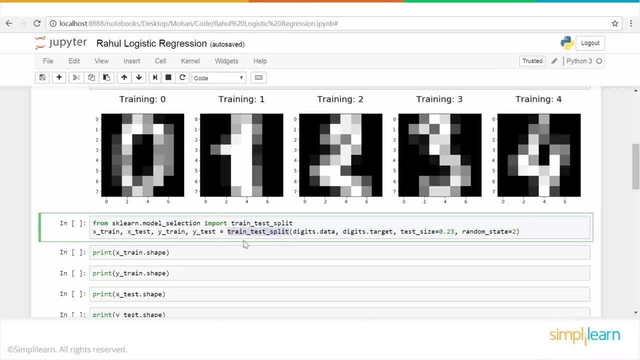 remaining 77 percent is used for training. remaining 77 percent is used for training. so there is a readily available function. so there is a readily available function. so there is a readily available function, which is which is which is called train test split. so we don't have 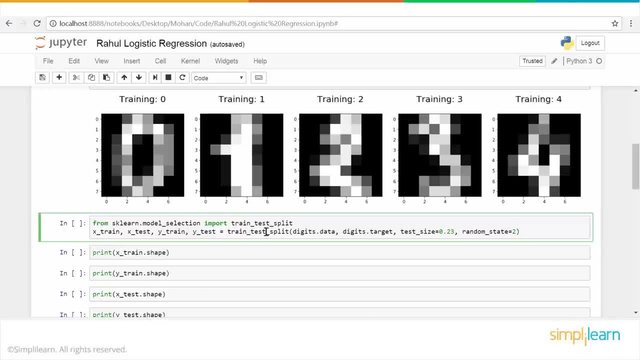 called train test split. so we don't have called train test split, so we don't have to write any special code for the. to write any special code for the. to write any special code for the: splitting- it will automatically split the splitting- it will automatically split the. 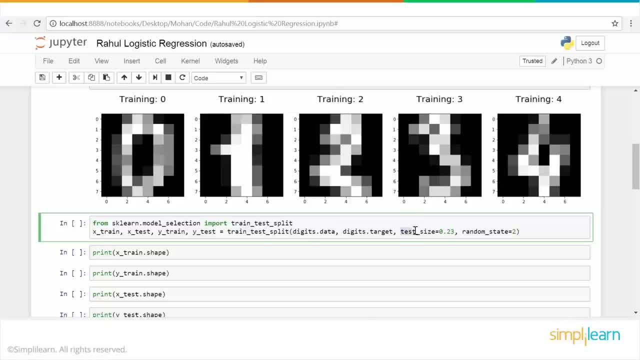 splitting. it will automatically split the data based on the proportion that we data, based on the proportion that we data, based on the proportion that we give here, which is test size, so we just give here which is test size, so we just give here which is test size, so we just the. the results will be stored in x. 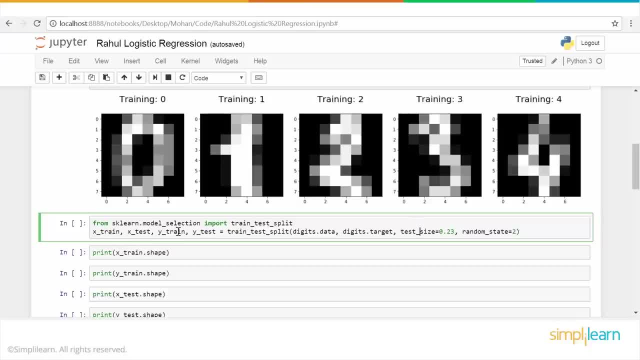 the- the results will be stored in x. the- the results will be stored in: x underscore train and y underscore train underscore train and y underscore train underscore train and y underscore train. for the training data set and what is x for the training data set and what is x. 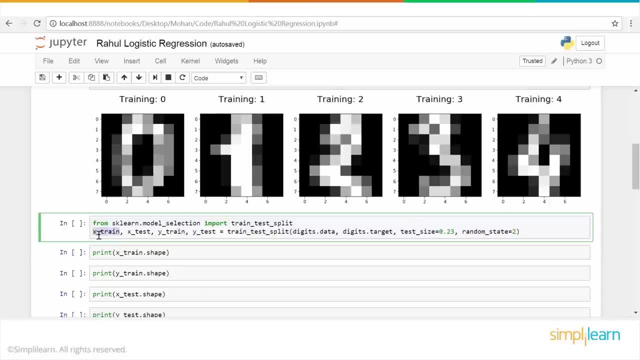 for the training data set. and what is x underscore train? this are: these are the underscore train. this are: these are the underscore train. this are these are the features. features, features, right, which is like the independent right, which is like the independent right, which is like the independent variable. 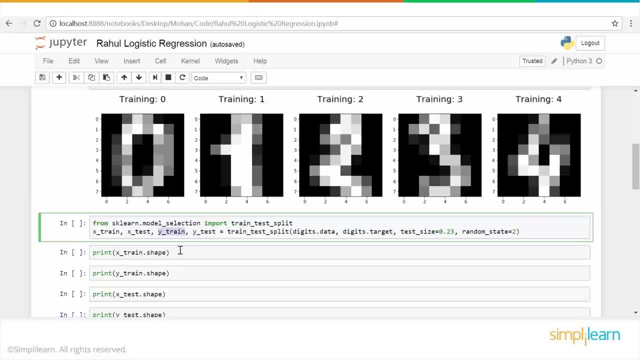 variable: variable and y underscore train is the label and y underscore train is the label and y underscore train is the label, right? so in this case, what happens, is we right? so in this case, what happens? is we right? so in this case, what happens is we have the input value, which is: or the 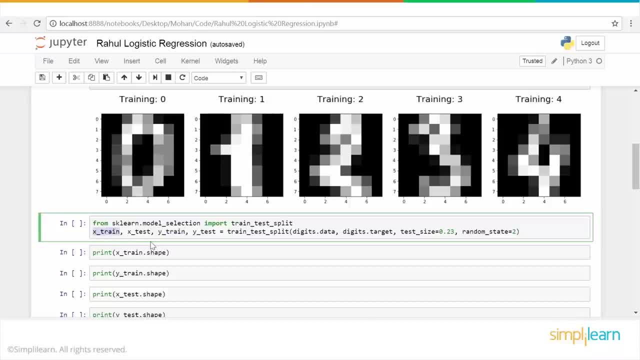 have the input value which is, or the have the input value which is, or the features value which is in x underscore features value which is in x underscore features value which is in x underscore train, and since this is the labeled data train, and since this is the labeled data, 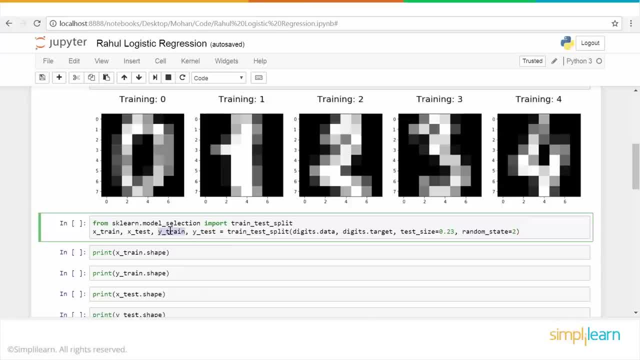 train and since this is the labeled data for each of them, each of the observations for each of them, each of the observations for each of them, each of the observations, we already have the label information. we already have the label information. we already have the label information saying whether this digit is a 0 or a 1. 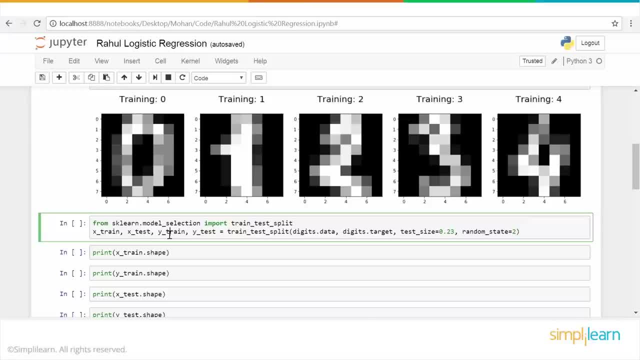 saying whether this digit is a 0 or a 1, saying whether this digit is a 0 or a 1 or a 2, so that that's this is what will. or a 2, so that that's this is what will. or a 2, so that that's this is what will be used for comparison to find out. 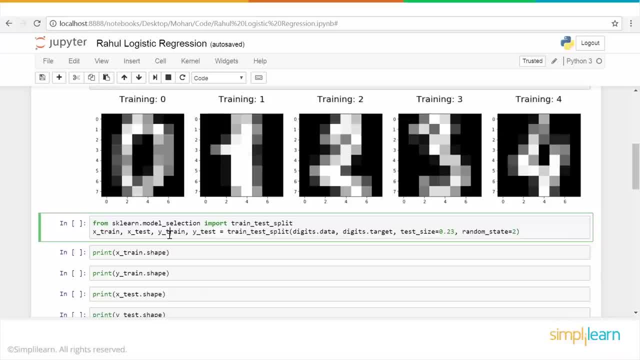 be used for comparison to find out. be used for comparison to find out whether the? the system is able to, whether the the system is able to, whether the the system is able to recognize it correctly, or there is an recognize it correctly, or there is an recognize it correctly or there is an error. for each observation, it will 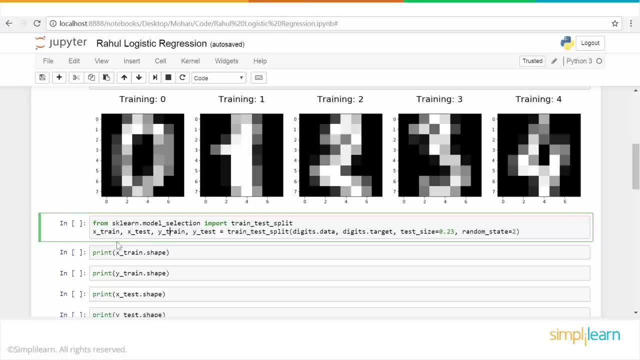 error for each observation. it will error for each observation. it will compare with this right. so this is the compare with this right. so this is the compare with this right. so this is the label. so the same way: x underscore train label. so the same way: x underscore train. 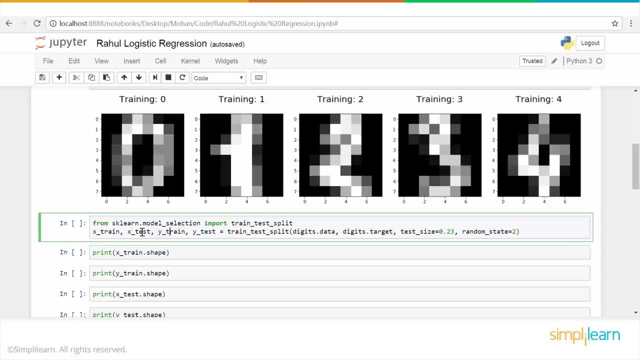 label. so the same way: x- underscore train. y underscore train is for the training, y underscore train is for the training, y underscore train is for the training data set. x underscore test. y underscore data set. x underscore test. y underscore data set. x underscore test. y underscore test is for the test data set. okay, so. 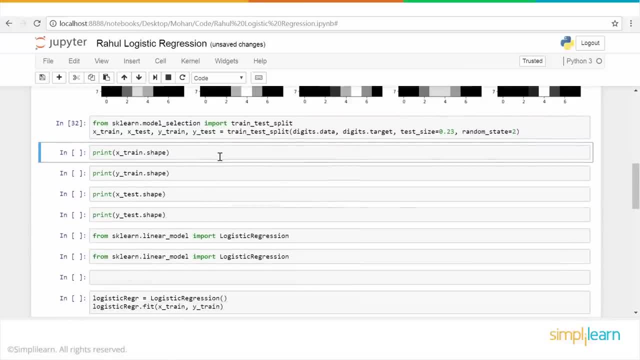 test is for the test data set. okay, so, test is for the test data set. okay. so let me go ahead and execute this code as. let me go ahead and execute this code as. let me go ahead and execute this code as well, and then we can go and check. 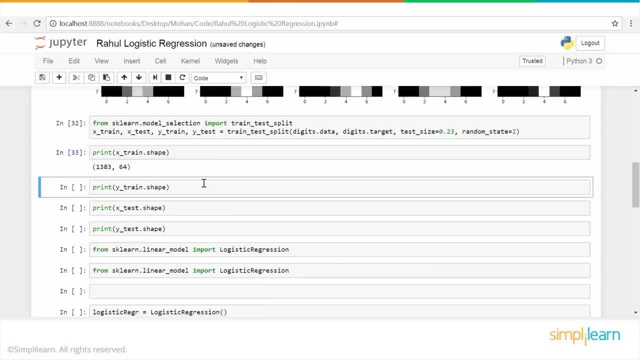 well, and then we can go and check well, and then we can go and check quickly. what is the how many entries are quickly? what is the how many entries are quickly? what is the how many entries are there, and in each of this, so x. there and in each of this, so x. 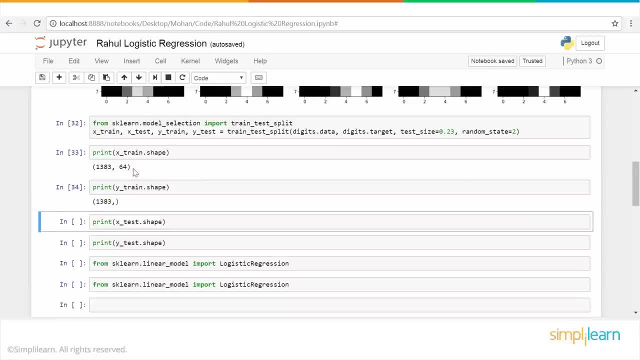 there and in each of this, so x. underscore train: the shape is 1383. underscore train: the shape is 1383. underscore train the shape is 1383 by 64 and y. underscore train has 1383 by 64 and y underscore train has 1383. 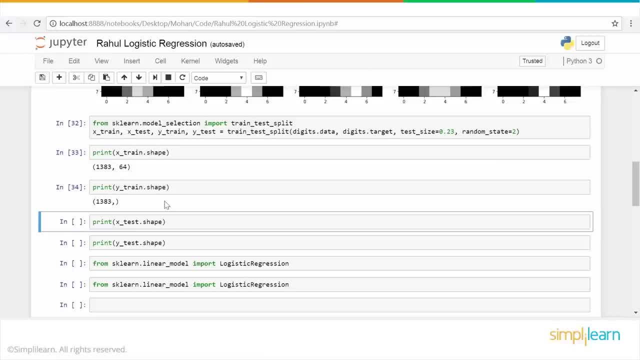 by 64 and y underscore train has 1383. because there is, because there is, because there is nothing like the second part is not nothing like the second part is not nothing like the second part is not required here. and then x underscore test required here, and then x underscore test. 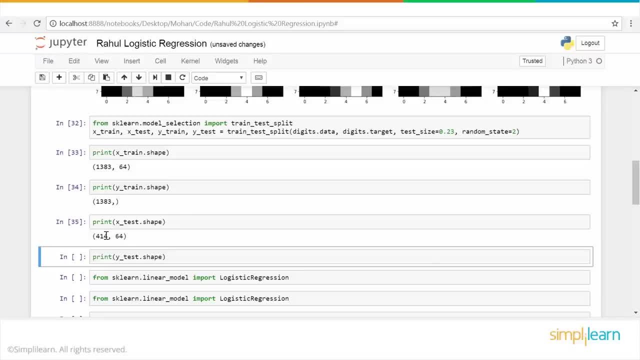 required here. and then x underscore test shape we see is 414. so actually there shape we see is 414. so actually there shape we see is 414. so actually there are 414 observations in test and 1383 are 414 observations in test and 1383. 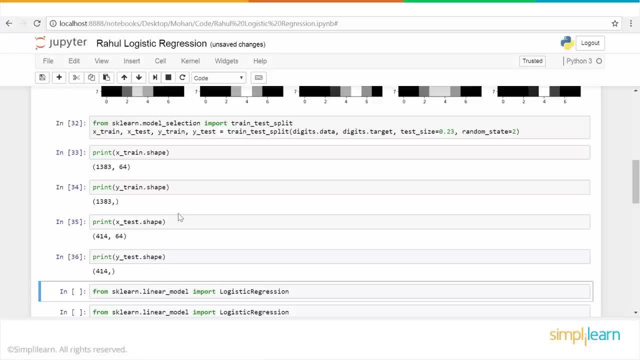 are 414 observations in test and 1383 observations in train. so that's basically observations in train. so that's basically observations in train. so that's basically what these four lines of code are saying. what these four lines of code are saying. what these four lines of code are saying: okay, then we import the logistic. 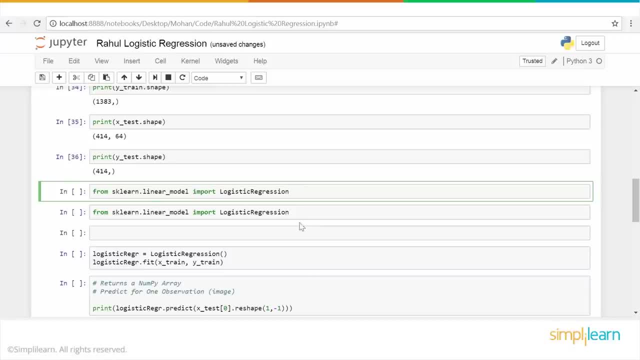 okay, then we import the logistic. okay, then we import the logistic, regression, regression, regression library, and which is a part of scikit library and which is a part of scikit library and which is a part of scikit learn so, learn so, learn, so we, we don't have to implement the. 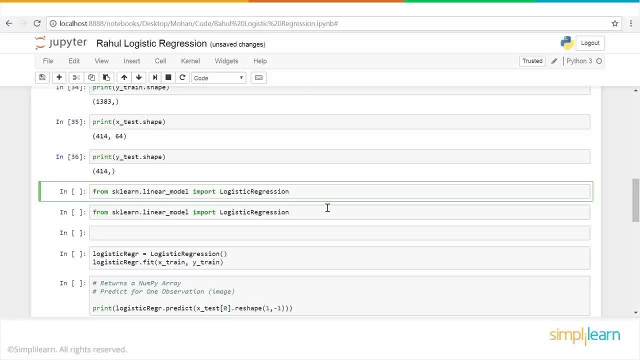 we, we don't have to implement the we, we don't have to implement the logistic regression process itself, we logistic regression process itself, we logistic regression process itself. we just call these, just call these, just call these the function, and let me go ahead and the function, and let me go ahead and 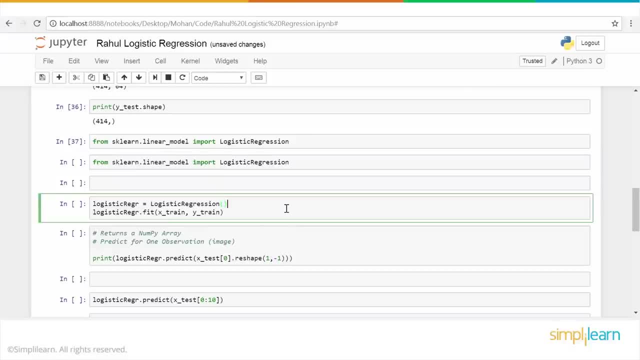 the function and let me go ahead and execute that so that. execute that, so that. execute that so that we have the logistic regression library. we have the logistic regression library, we have the logistic regression library imported. now we create an instance of imported. now we create an instance of. 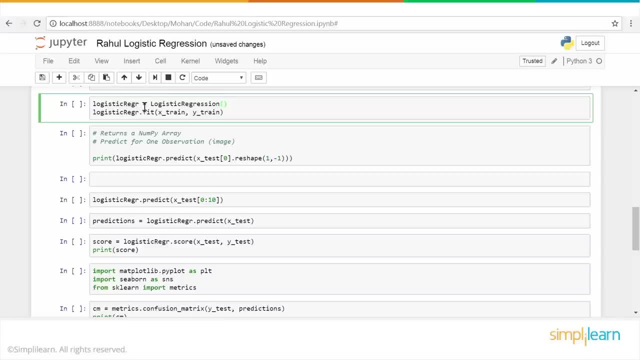 imported. now we create an instance of logistic regression. right so logistic regression, right so logistic regression, right so logistic regr is a is an instance of logistic regr is a is an instance of logistic regr is a is an instance of logistic regression, logistic regression, logistic regression- an instance of logistic regression model. 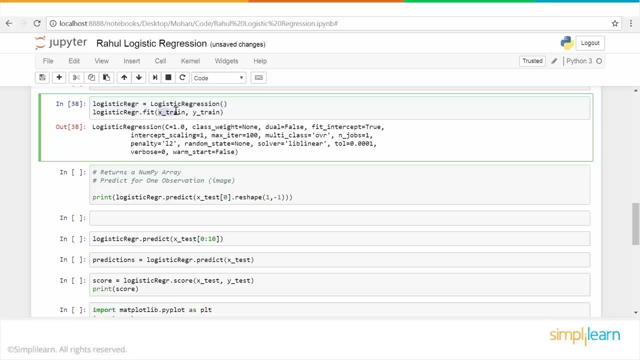 an instance of logistic regression model. an instance of logistic regression model. and then the second line way is where we, and then the second line way is where we, and then the second line way is where we are passing, are passing, are passing our data, the training data set and this. 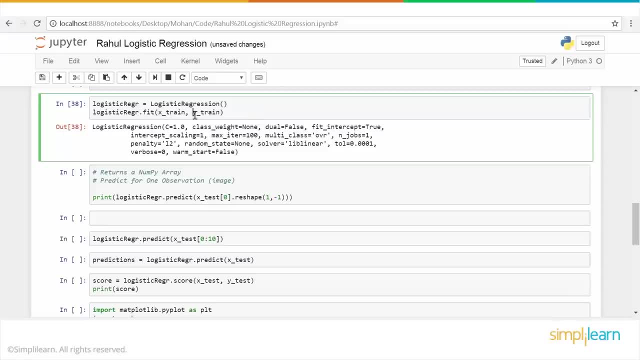 our data, the training data set, and this, our data, the training data set, and this is our, is our, is our the predictors and uh, this is our target. the predictors and uh, this is our target. the predictors and uh, this is our target. we are passing this data set. 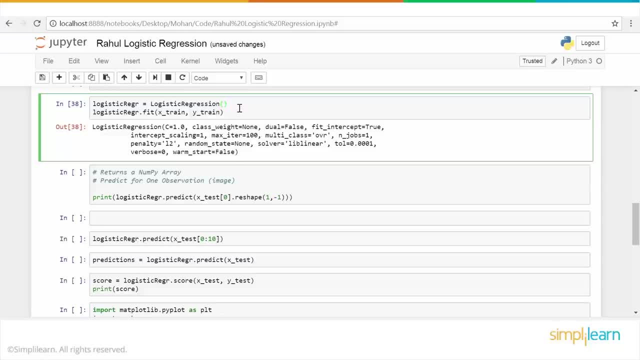 we are passing this data set. we are passing this data set to train our model. all right, so to train our model. all right, so to train our model, all right. so, once we do this, in this case, the data. once we do this, in this case, the data- 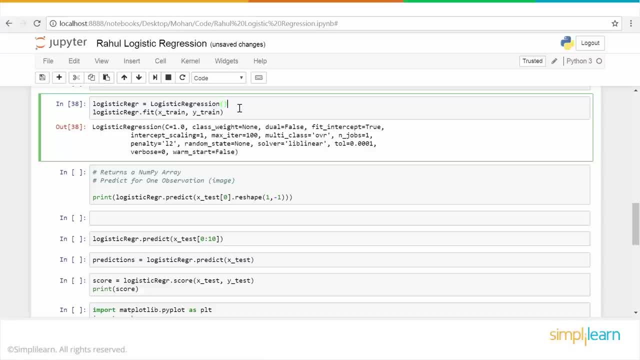 once we do this. in this case, the data is not large but is not large, but we spend a lot of time for the training. we spend a lot of time for the training. we spend a lot of time for the training. part of it, part of it, part of it. okay, so here the data set is relatively 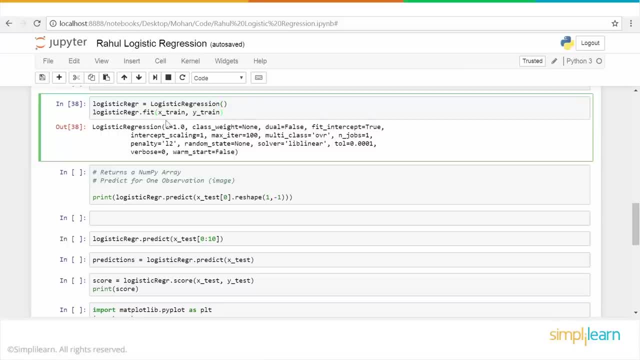 okay. so here the data set is relatively okay. so here the data set is relatively small. so it was pretty quick. so all small, so it was pretty quick, so all small, so it was pretty quick, so all right. so now our right. so now our right. so now our model has been trained using the. 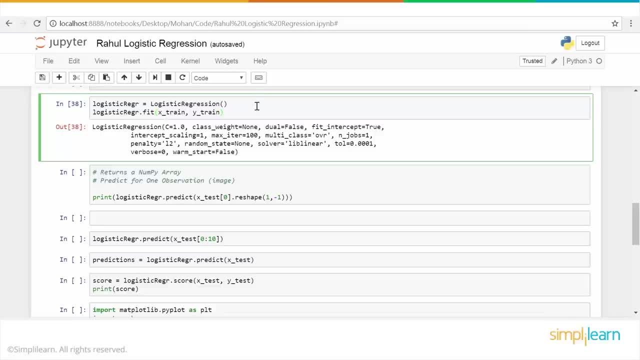 model has been trained using. the model has been trained using the training data set, training data set, training data set- and we want to see how accurate this is, and we want to see how accurate this is, and we want to see how accurate this is. so what we'll do is we will test it out. 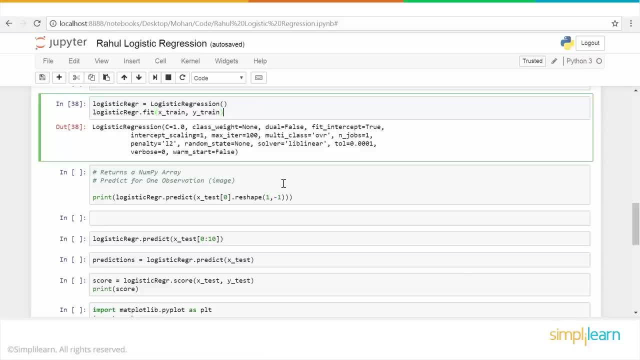 so what we'll do is: we will test it out. so what we'll do is we will test it out in probably faces. so let me first try in probably faces. so let me first try in probably faces. so let me first try out how well this is working for one. 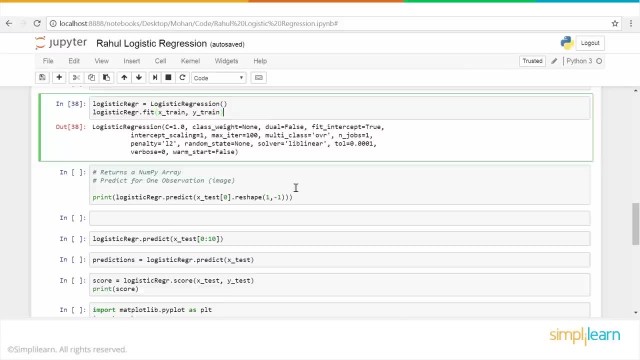 out how well this is working for one, out how well this is working for one image. okay, i will just try it out with image. okay, i will just try it out with image. okay, i will just try it out with one image, my one image, my one image, my the first entry in my test data set and 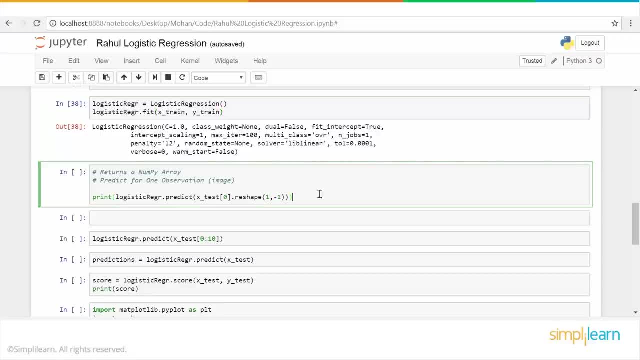 the first entry in my test data set and the first entry in my test data set and see whether it is, see whether it is see whether it is correctly predicting or not so, and in correctly predicting or not so, and in correctly predicting or not so, and in order to test it. 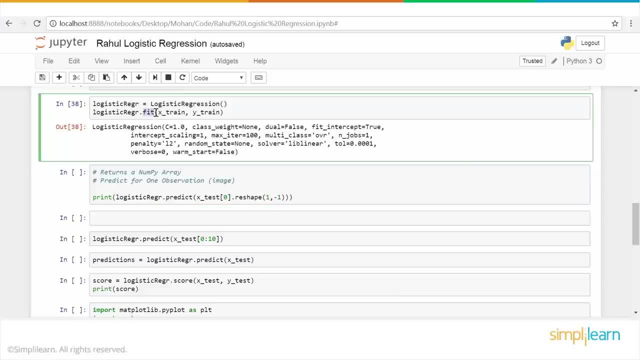 order to test it, order to test it, so for training purpose, we use the fit. so for training purpose, we use the fit. so for training purpose, we use the fit method. there is a method called fit method, there is a method called fit method, there is a method called fit, which is for training the model, and once. 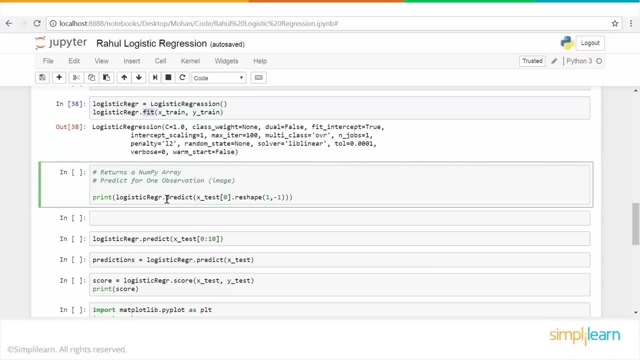 which is for training the model and once which is for training the model and once the training is done. if you want to test, the training is done. if you want to test, the training is done. if you want to test for a particular value- new input- you use. 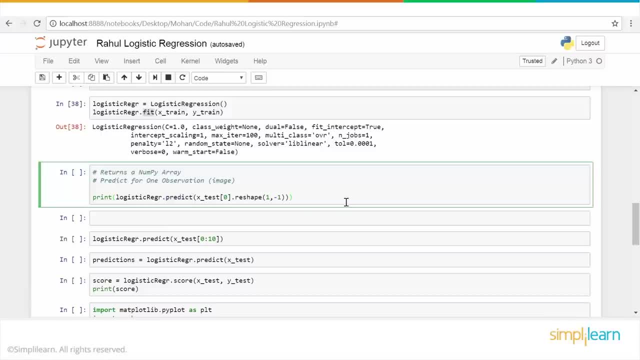 for a particular value: new input. you use for a particular value: new input. you use the predict method. okay, so let's run the- the predict method. okay, so let's run the- the predict method. okay, so let's run the predict method and we pass this predict method and we pass this. 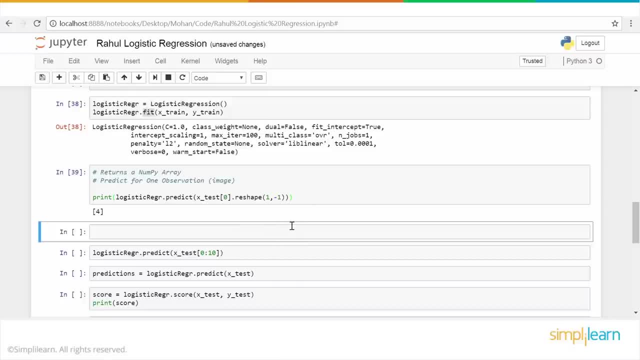 predict method and we pass this particular image and particular image and particular image and we see that the shape is or the. we see that the shape is or the. we see that the shape is or. the prediction is four, so let's try a few. prediction is four, so let's try a few. 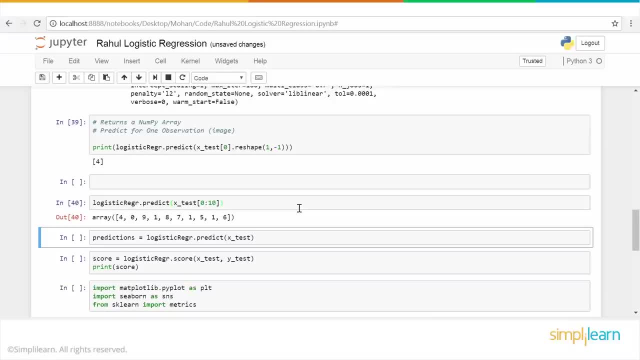 prediction is four, so let's try a few more. let me see for the next 10. seems to more. let me see for the next 10. seems to more. let me see for the next 10. seems to be fine, so let me just go ahead and. 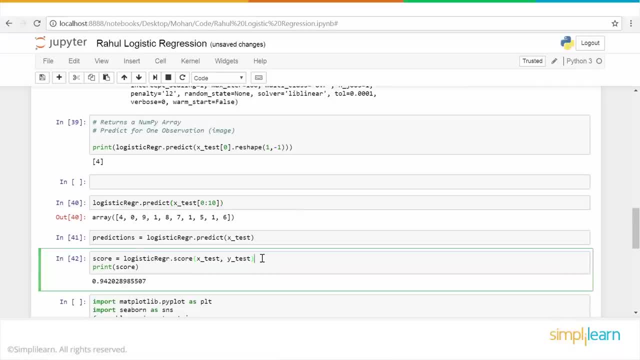 be fine, so let me just go ahead and be fine. so let me just go ahead and test the entire data set. okay, that's test the entire data set. okay, that's test the entire data set. okay, that's basically what we will do. so now we want: 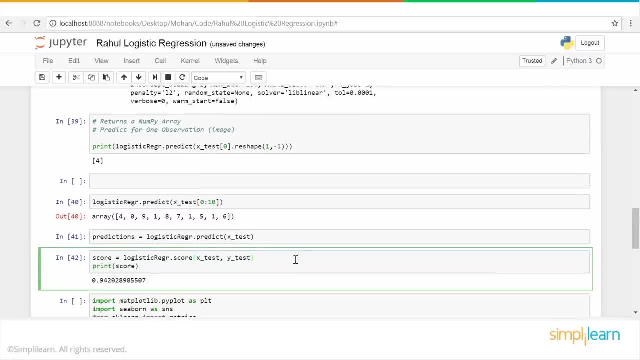 basically what we will do so now. we want basically what we will do so now. we want to find out how accurately this has to find out how accurately this has to find out how accurately this has performed. so we use the score method to performed. so we use the score method to. 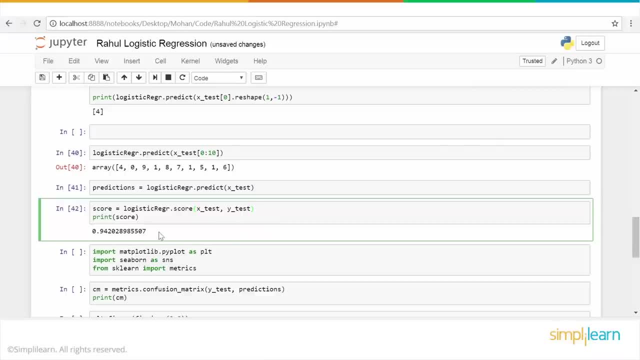 performed. so we use the score method to find what is the percentage of accuracy. find what is the percentage of accuracy, find what is the percentage of accuracy. and we see here that it has performed up. and we see here that it has performed up, and we see here that it has performed up to 94 percent accurate. okay, so that's on. 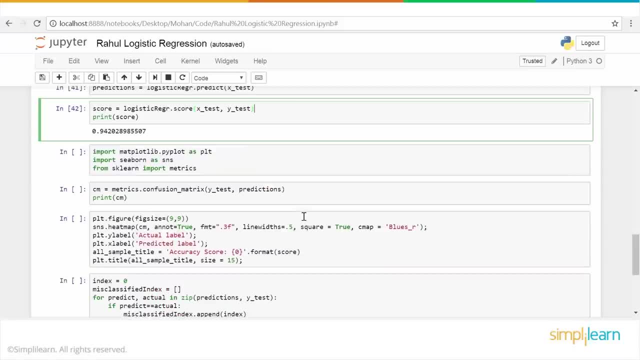 to 94 percent accurate. okay, so that's on to 94 percent accurate, okay. so that's on this part now. what we can also do is we this part now. what we can also do is we this part now. what we can also do is: we can also see this accuracy using what is. 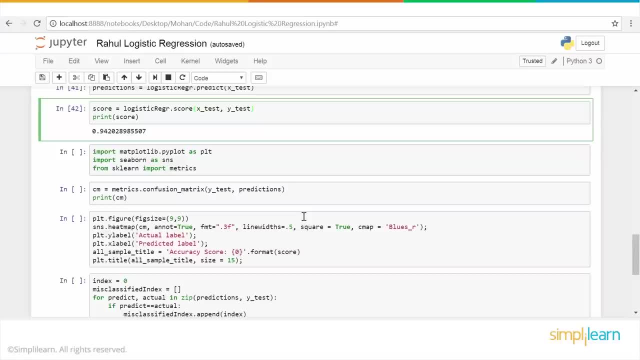 can also see this accuracy using what is. can also see this accuracy using what is known as a confusion matrix. so let us go. known as a confusion matrix, so let us go. known as a confusion matrix, so let us go ahead and try that as well, so that we 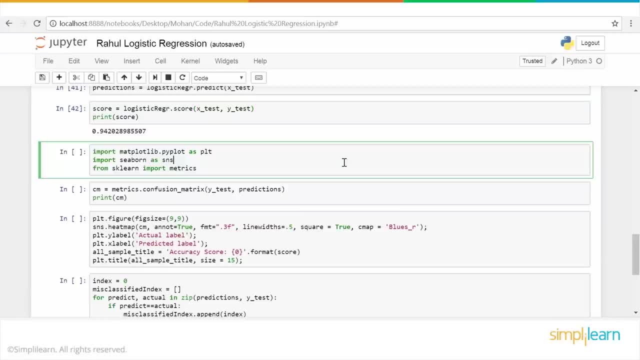 ahead and try that as well, so that we ahead and try that as well, so that we can also visualize how well this model can also visualize, how well this model can also visualize how well this model has done so let me execute this piece of. has done so. let me execute this piece of. 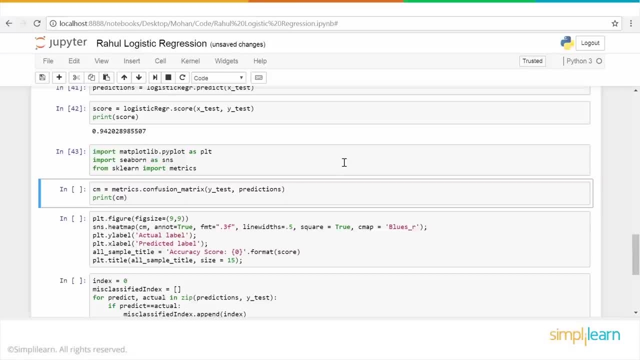 has done so. let me execute this piece of code, which will basically import some of code, which will basically import some of code, which will basically import some of the libraries that are required and the libraries that are required, and the libraries that are required, and we we basically create a confusion matrix. 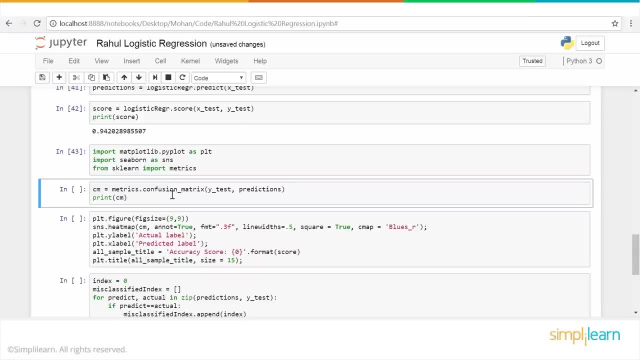 we we basically create a confusion matrix. we we basically create a confusion matrix and instance of confusion matrix by and instance of confusion matrix by and instance of confusion matrix by running confusion matrix and passing running confusion matrix and passing running confusion matrix and passing these values. so we have, so this: 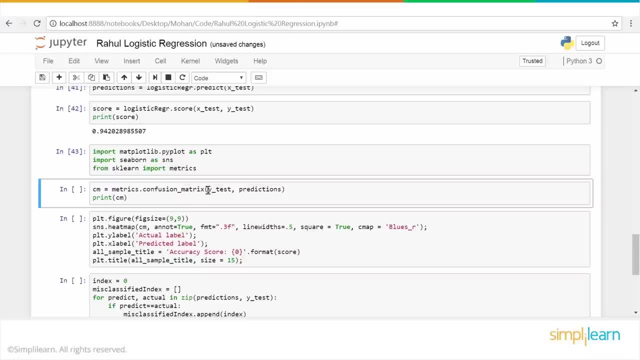 these values, so we have so this, these values, so we have, so this confusion. underscore matrix method takes confusion. underscore matrix method takes confusion. underscore matrix method takes two parameters. one is the y underscore. two parameters, one is the y underscore. two parameters: one is the y underscore test and the other is the prediction. so 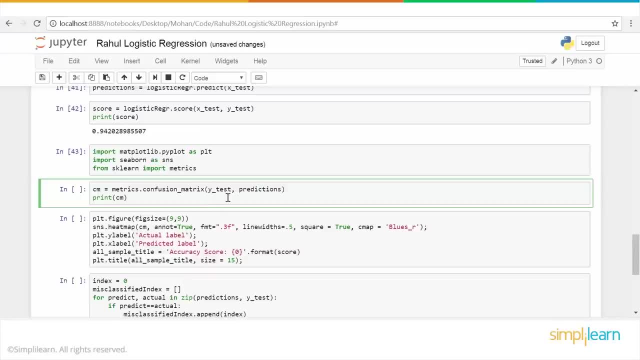 test and the other is the prediction. so test and the other is the prediction. so what is the y underscore test? these are: what is the y underscore test. these are: what is the y underscore test. these are the labeled values which we already know. the labeled values which we already know. 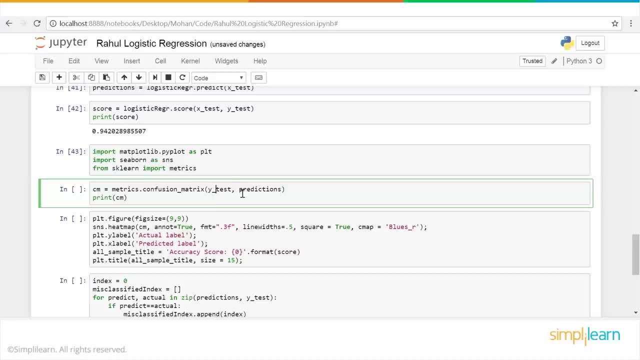 the labeled values which we already know for the test data set and predictions for the test data set and predictions for the test data set and predictions are what the system has predicted for. are what the system has predicted for. are what the system has predicted for the test data set. okay, so this is known. 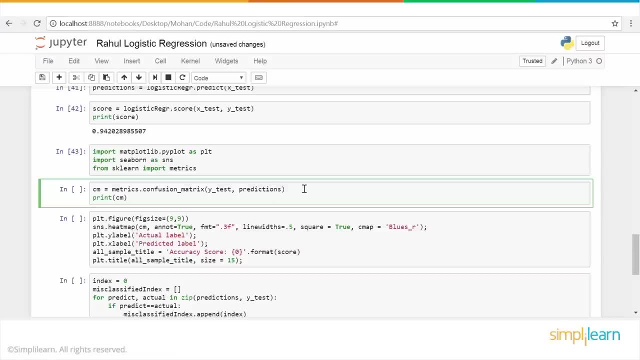 the test data set: okay, so this is known. the test data set: okay, so this is known to us, to us, to us, and this is what the system has, and this is what the system has, and this is what the system has the model has generated. so we kind of 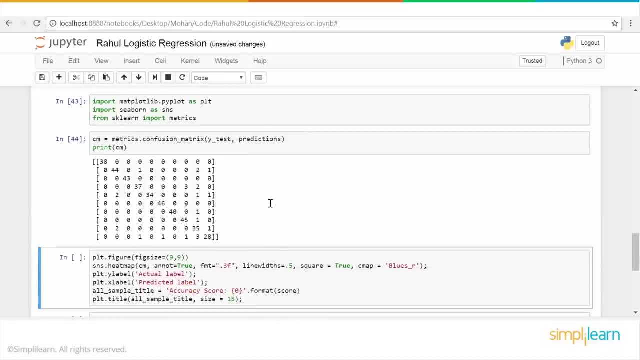 the model has generated. so we kind of the model has generated, so we kind of create the confusion matrix and we will create the confusion matrix and we will create the confusion matrix and we will print it. and this is how the confusion print it and this is how the confusion. 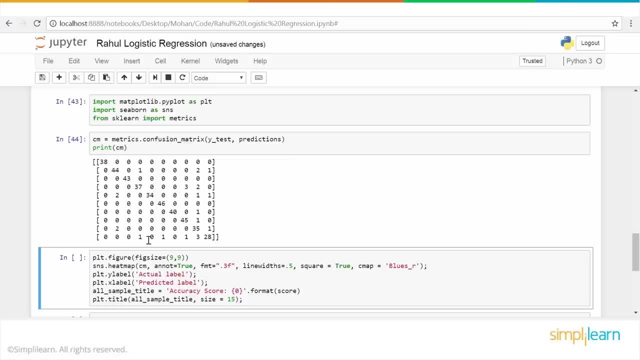 print it, and this is how the confusion: matrix looks as the name suggests it is. matrix looks as the name suggests it is. matrix looks as the name suggests: it is a matrix, a matrix, a matrix, and, and. and the key point out here is that the the key point out here is that the 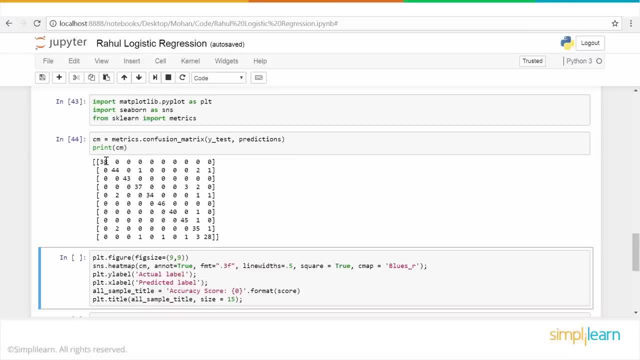 the key point out here is that the accuracy of the model is determined by. accuracy of the model is determined by. accuracy of the model is determined by how many numbers are there in the. how many numbers are there in the? how many numbers are there in the diagonal? the more the numbers in the. 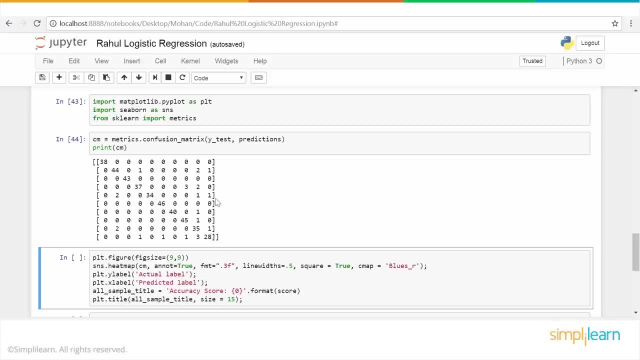 diagonal. the more the numbers in the diagonal, the more the numbers in the diagonal, the better the accuracy is diagonal. the better the accuracy is diagonal, the better the accuracy is okay and first of all, the total sum of okay and first of all the total sum of okay and first of all the total sum of all the numbers in this whole matrix is: 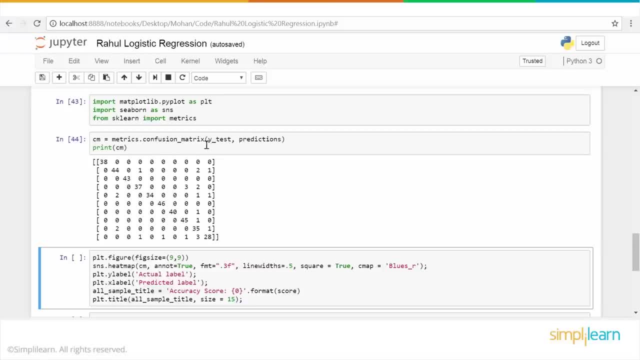 all the numbers in this whole matrix, is all the numbers in this whole matrix is equal to the number of observations in, equal to the number of observations in, equal to the number of observations in the test data set. that is the first. the test data set. that is the first. 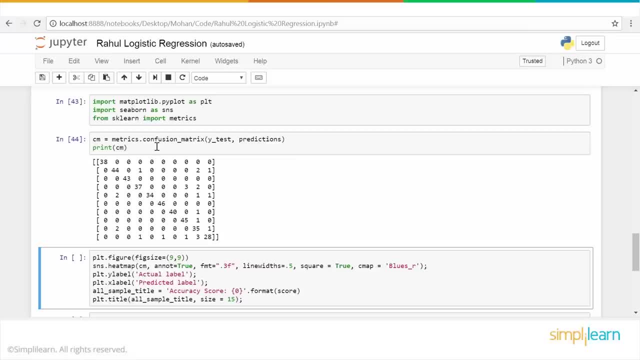 the test data set. that is the first thing, right? so if you add up all these thing, right? so, if you add up all these thing, right? so if you add up all these numbers, that will be equal to the number, numbers that will be equal to the number. 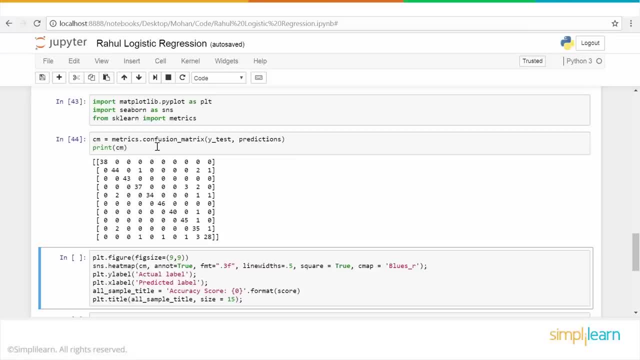 numbers that will be equal to the number of, of, of observations in the test data set and observations in the test data set and observations in the test data set and then out of that, the maximum number of, then out of that, the maximum number of, then out of that, the maximum number of them should be in the diagonal that. 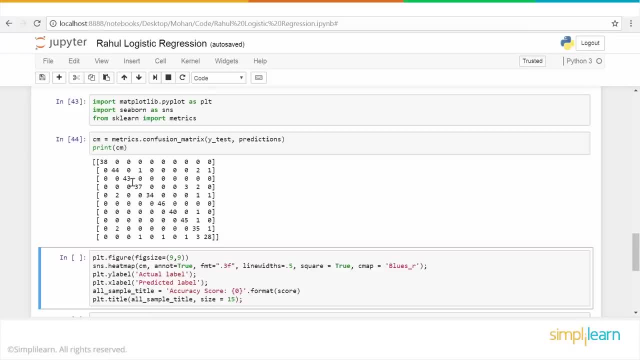 them should be in the diagonal, that them should be in the diagonal, that means the accuracy is pretty good. if means the accuracy is pretty good. if means the accuracy is pretty good if the- the numbers in the diagonal are less, the- the numbers in the diagonal are less. 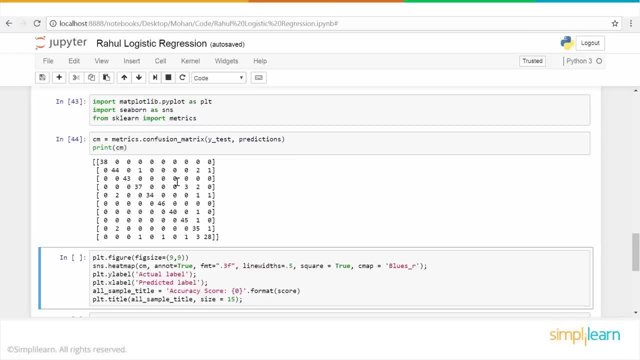 the, the numbers in the diagonal are less, and in all other places there are a lot, and in all other places there are a lot, and in all other places there are a lot of numbers, of numbers, of numbers, which means the accuracy is very low. the, which means the accuracy is very low. the. 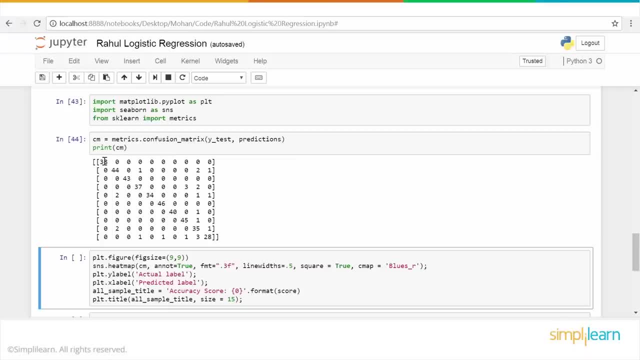 which means the accuracy is very low. the diagonal indicates a correct prediction. diagonal indicates a correct prediction. diagonal indicates a correct prediction that this means that the actual value is that this means that the actual value is that this means that the actual value is same as the predicted value. here again, 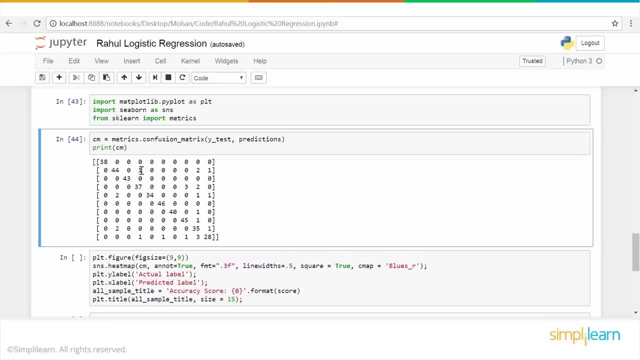 same as the predicted value. here again, same as the predicted value. here again, actual value same as a predictive value. actual value, same as a predictive value. actual value same as a predictive value, and so on. right, so the moment you see a, and so on. right, so the moment you see a. 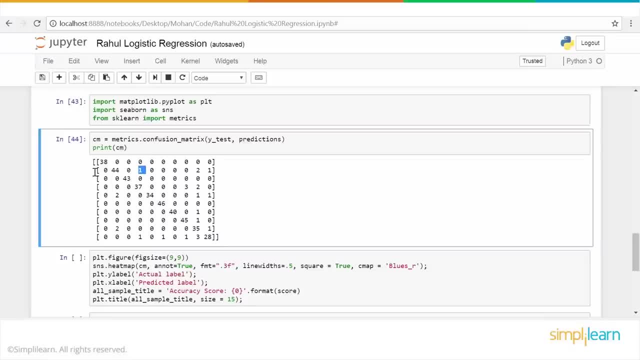 and so on. right, so the moment you see a number here, that means the actual value number here, that means the actual value number here. that means the actual value is something and the predicted value is is something, and the predicted value is is something and the predicted value is something else. right? similarly, here the 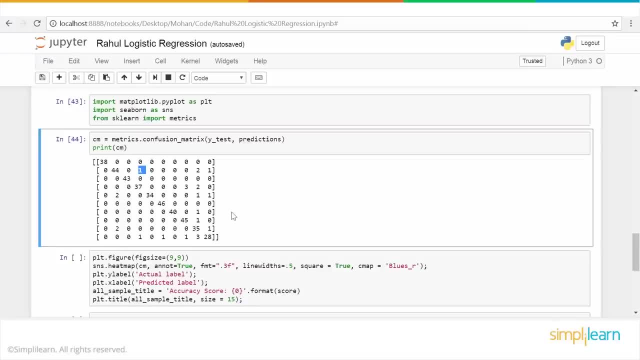 something else right. similarly here, the something else right. similarly here. the actual value is something and the actual value is something, and the actual value is something and the predicted value is something else. so predicted value is something else, so predicted value is something else. so that is basically how we read the. 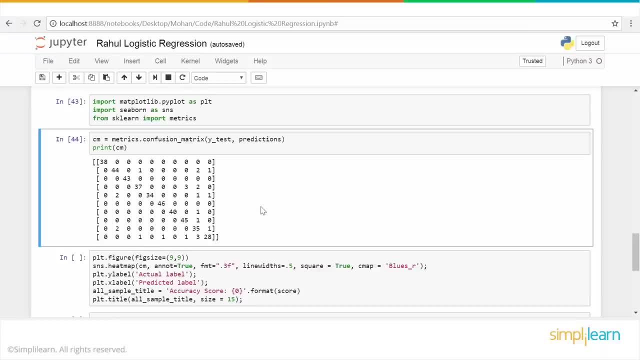 that is basically how we read the. that is basically how we read the confusion matrix. now, how do we find the confusion matrix now? how do we find the confusion matrix now? how do we find the accuracy? you can actually add up the accuracy. you can actually add up the. 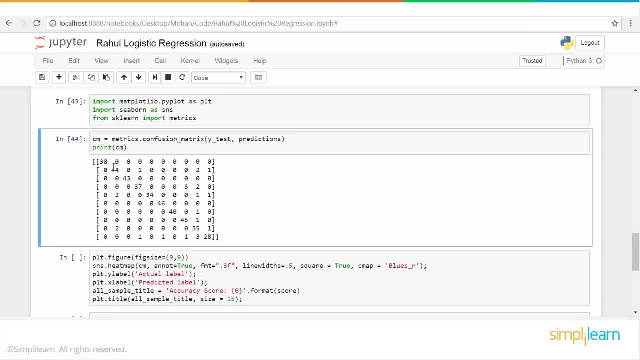 accuracy, you can actually add up the total values in the diagonal. so it's total values in the diagonal, so it's total values in the diagonal, so it's like 38 plus 44 plus 43 and so on, and like 38 plus 44 plus 43 and so on, and 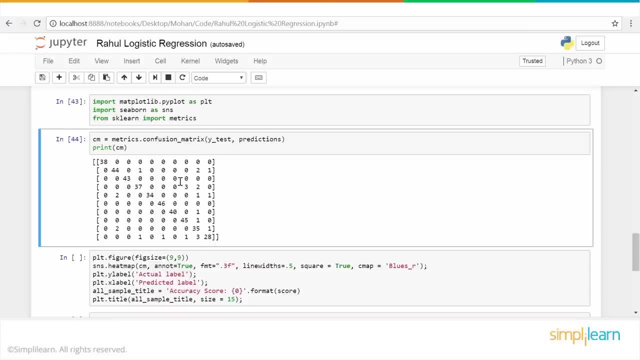 like 38 plus 44 plus 43 and so on, and divide that by the total number of test. divide that by the total number of test. divide that by the total number of test observations. that will give you the observations. that will give you the observations that will give you the percentage accuracy. using a confusion. 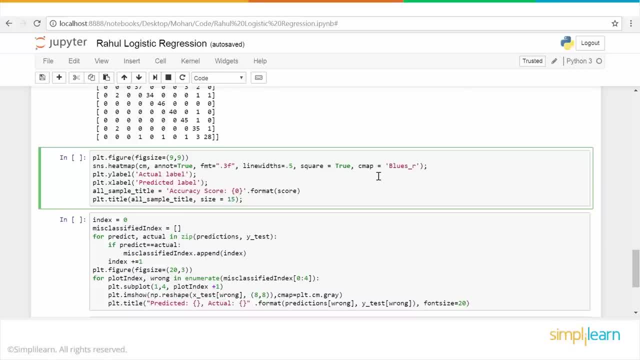 percentage accuracy using a confusion percentage accuracy using a confusion matrix. now, let us visualize this matrix now. let us visualize this matrix now. let us visualize this confusion matrix in a slightly more confusion matrix, in a slightly more confusion matrix, in a slightly more sophisticated way, using a heat map. so we 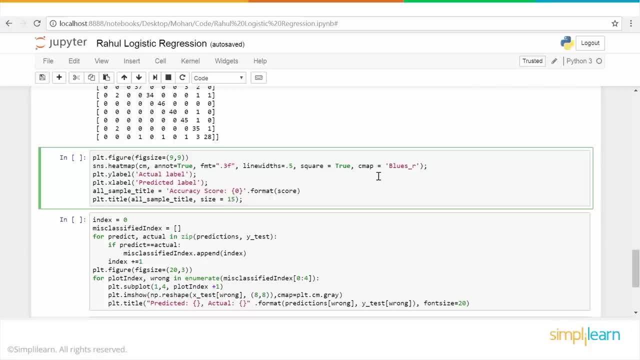 sophisticated way using a heat map. so we sophisticated way using a heat map, so we will create a heat map with some. we'll will create a heat map with some. we'll will create a heat map with some. we'll add some colors as well. it's, uh, it's. 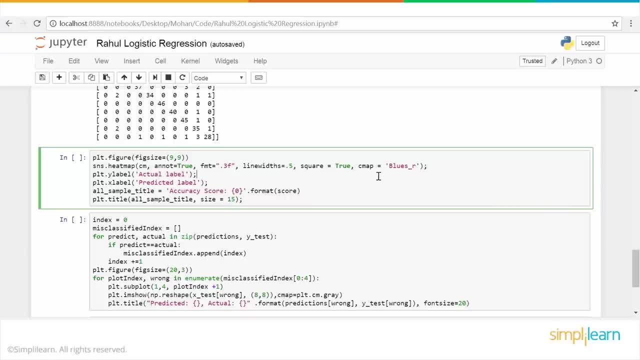 add some colors as well. it's, uh, it's, add some colors as well. it's, uh, it's like a more visually visually more, like a more visually visually more, like a more visually visually more appealing. so that's the whole idea. so if appealing, so that's the whole idea. so if 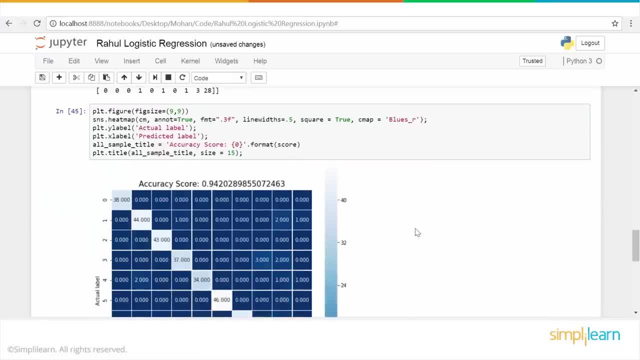 appealing. so that's the whole idea. so, if we let me run this piece of code and we let me run this piece of code and we let me run this piece of code, and this is how the heat map looks, and as. this is how the heat map looks and as. 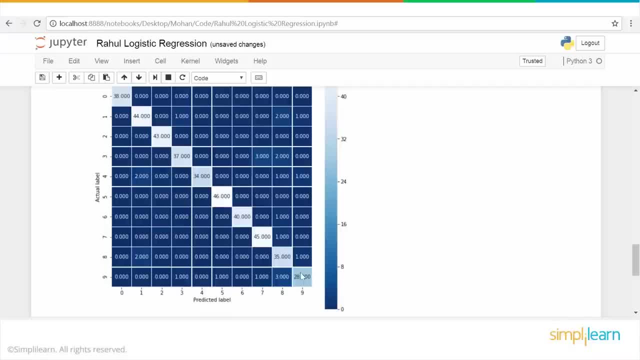 this is how the heat map looks and, as you can see here the diagonals again. you can see here the diagonals again. you can see here the diagonals again: are all the values are here most of the. are all the values are here, most of the. 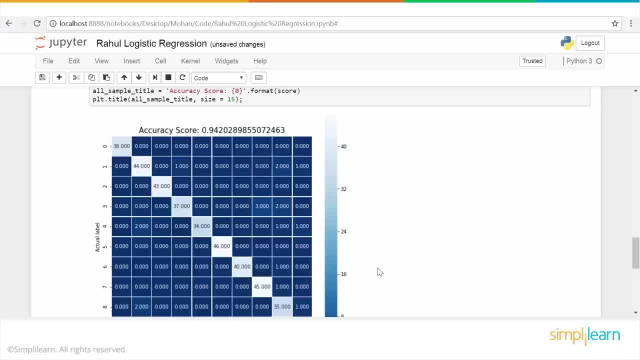 are all the values are here, most of the values. so, which means reasonably this values. so which means reasonably this values. so which means reasonably, this seems to be reasonably accurate and yeah, seems to be reasonably accurate. and yeah, seems to be reasonably accurate and yeah, basically the accuracy score is 94. this. 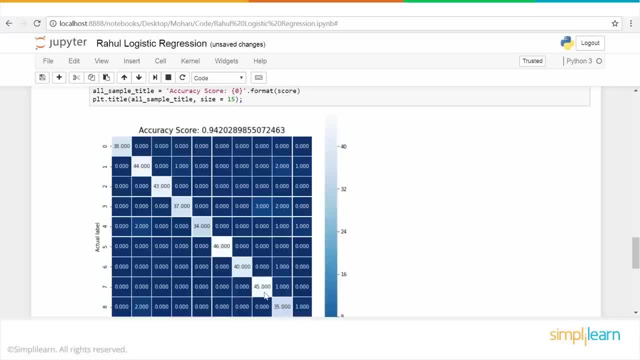 basically, the accuracy score is 94. this, basically, the accuracy score is 94. this is calculated, as i mentioned, by adding. is calculated, as i mentioned, by adding. is calculated, as i mentioned, by adding all these numbers divided by the total, all these numbers divided by the total. 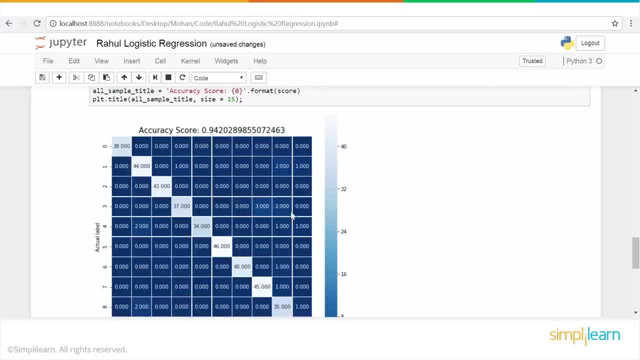 all these numbers divided by the total test values, or the total number of test values, or the total number of test values, or the total number of observations in test data set. observations in test data set. observations in test data set. okay, so this is the confusion matrix for. 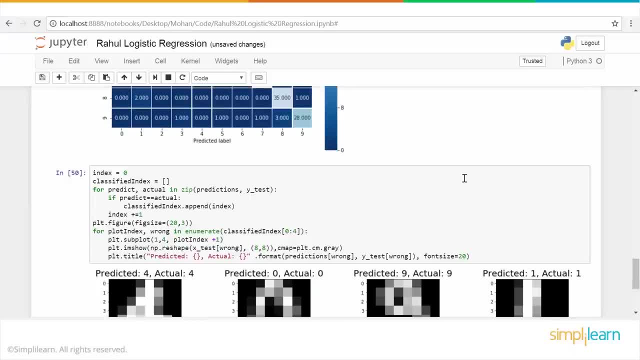 okay, so this is the confusion matrix for okay, so this is the confusion matrix for logistic regression: logistic regression, logistic regression, all right. so, now that we have seen the all right, so now that we have seen the all right, so now that we have seen the confusion matrix, let's take a quick. 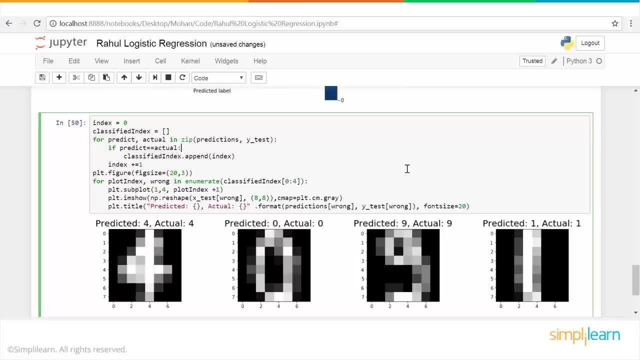 confusion matrix. let's take a quick confusion matrix. let's take a quick sample and see how well the system has sample and see how well the system has sample and see how well the system has classified and we will take a few classified and we will take a few. 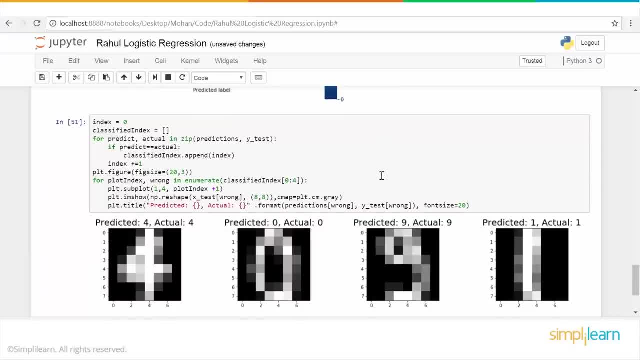 classified and we will take a few examples of the data. so if we see here examples of the data, so if we see here examples of the data, so if we see here we we picked up randomly a few of them, we we picked up randomly a few of them. 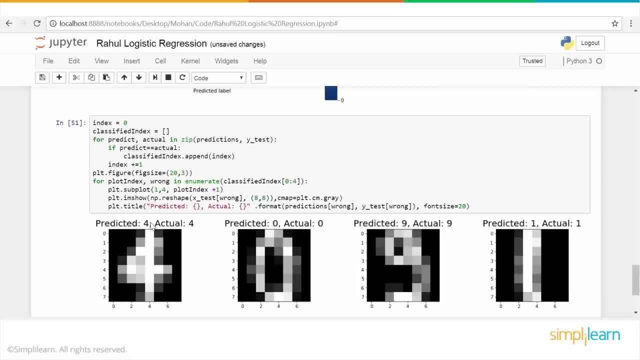 we. we picked up randomly a few of them. so this is uh number four, which is the. so this is uh number four, which is the. so this is uh number four, which is the actual value and also the predicted actual value, and also the predicted actual value and also the predicted value. both are four. 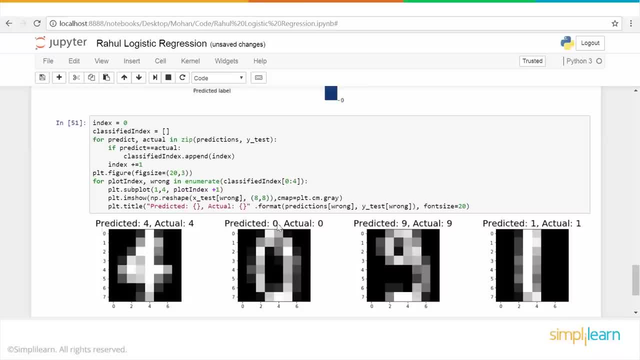 value: both are four. value: both are four. this is an image of zero. so the predicted: this is an image of zero. so the predicted: this is an image of zero. so the predicted value is also zero. actual values of value is also zero. actual values of value is also zero. actual values, of course, zero. 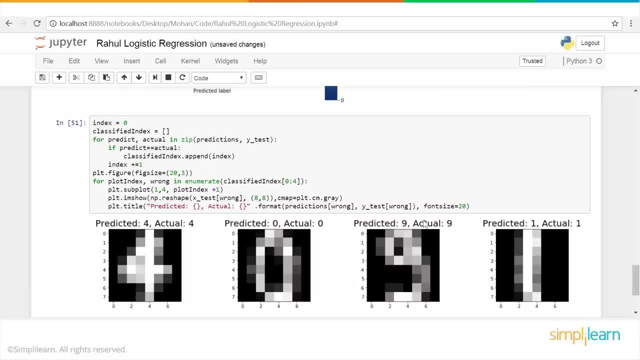 course, zero, course, zero. then this is the image of nine, then this is the image of nine, then this is the image of nine. so this has also been predicted, so this has also been predicted. so this has also been predicted correctly. nine and actual value is nine. correctly: nine and actual value is nine. 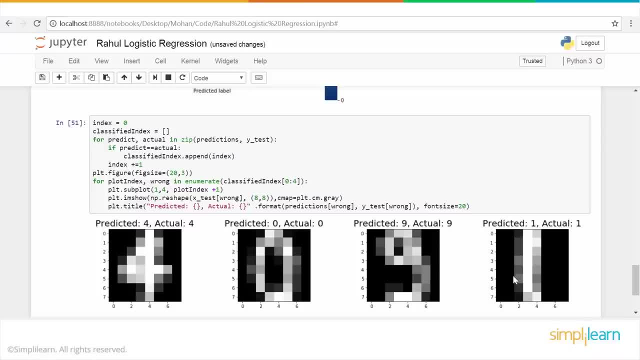 correctly nine and actual value is nine, and this is the image of one and again, and this is the image of one and again, and this is the image of one and again. this has been predicted correctly. as this has been predicted correctly, as this has been predicted correctly as like the actual value. okay, so this was a. 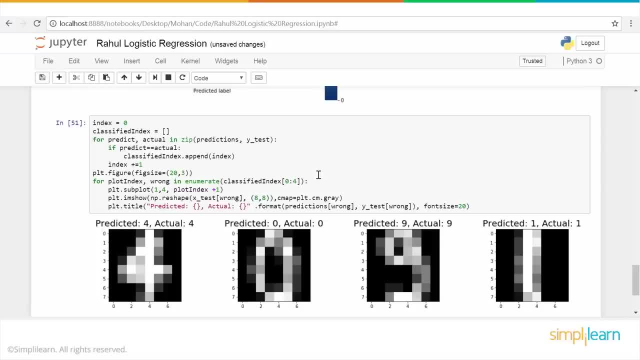 like the actual value. okay, so this was a like the actual value. okay, so this was a quick demo of quick demo of quick demo of logistic regression: how to use logistic logistic regression. how to use logistic logistic regression. how to use logistic regression to regression to regression to identify images. okay, 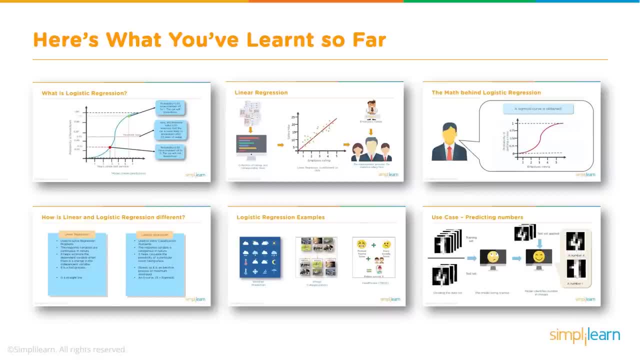 identify images, okay, identify images, okay. so let's summarize what we have. so let's summarize what we have. so let's summarize what we have learned in this video. we discussed about learned in this video. we discussed about learned in this video. we discussed about what is logistic regression and how it. 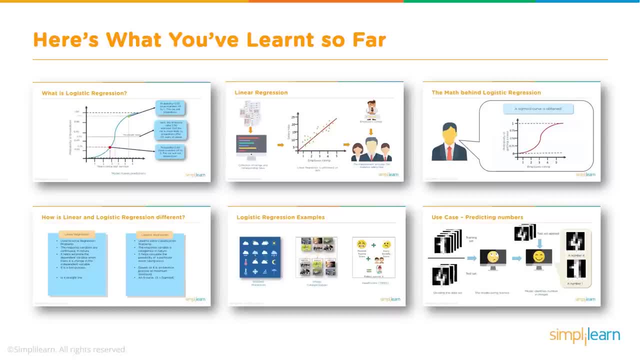 what is logistic regression and how it? what is logistic regression and how it fits into the overall machine learning? fits into the overall machine learning, fits into the overall machine learning. we discussed about the different types. we discussed about the different types. we discussed about the different types of machine learning and how logistic 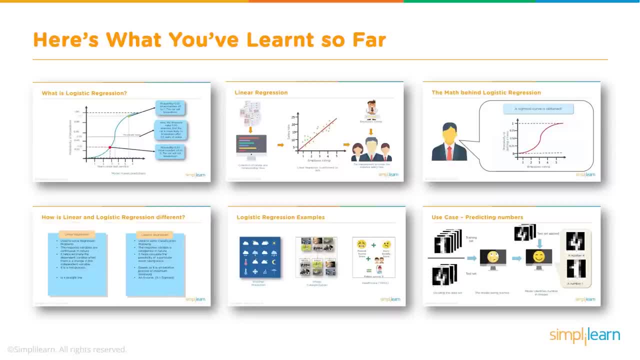 of machine learning and how logistic of machine learning and how logistic regression is one of the algorithms for regression, is one of the algorithms for regression, is one of the algorithms for classification. and then we compared classification, and then we compared classification and then we compared logistic regression with linear. 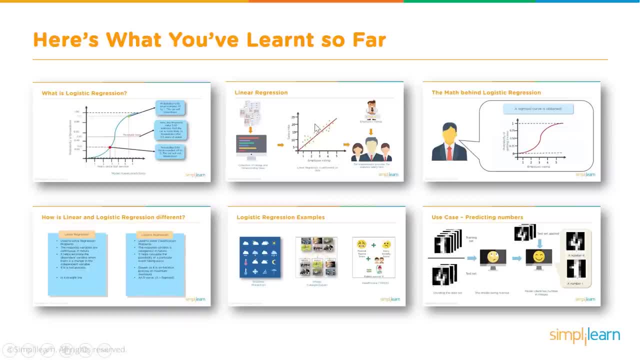 logistic regression with linear logistic regression, with linear regression, because the names may be regression, because the names may be regression, because the names may be sounding similar, but these are completely sounding similar, but these are completely sounding similar, but these are completely different algorithms linear regression, different algorithms: linear regression. 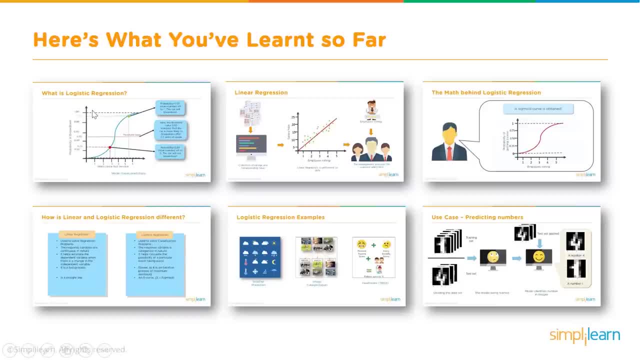 different algorithms. linear regression is used for predicting continuous values, is used for predicting continuous values, is used for predicting continuous values, whereas logistic regression is used for, whereas logistic regression is used for, whereas logistic regression is used for finding discrete values. and then we finding discrete values, and then we. 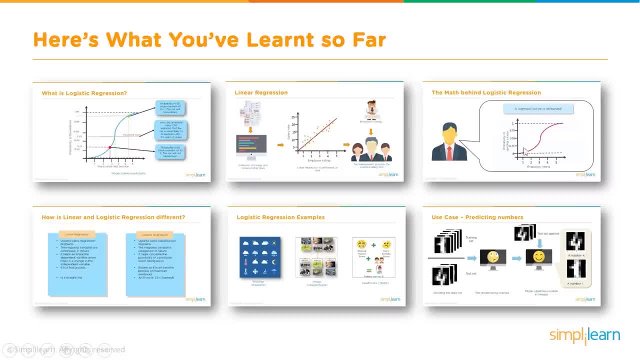 finding discrete values. and then we talked about the math behind logistic, talked about the math behind logistic, talked about the math behind logistic regression and we derived that function regression and we derived that function regression and we derived that function as well. the sigmoid function. we did a. as well, the sigmoid function, we did a. 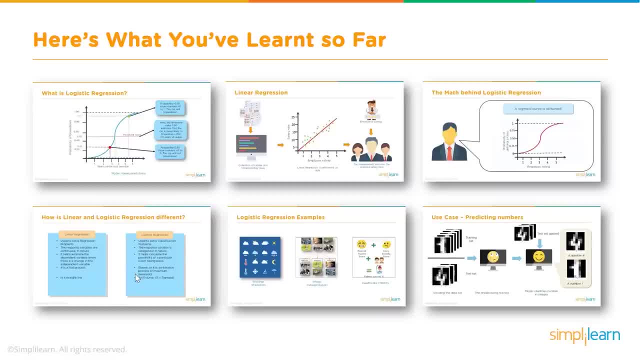 as well the sigmoid function. we did a quick tabular comparison between linear. quick tabular comparison between linear. quick tabular comparison between linear and logistic regression. we saw some and logistic regression: we saw some. and logistic regression: we saw some examples of day-to-day life how logistic. 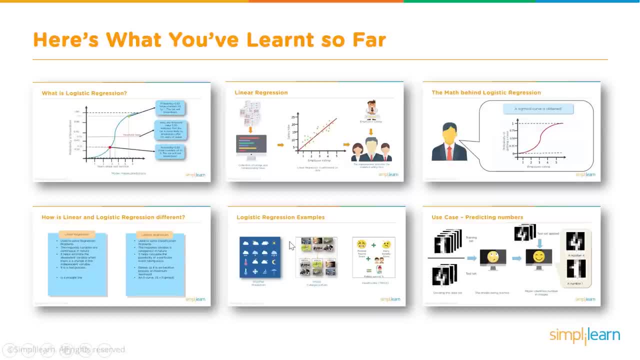 examples of day-to-day life. how logistic examples of day-to-day life. how logistic regression is used for some of the regression is used for some of the regression is used for some of the class for solving some of the class for solving some of the class for solving some of the classification problems and then in the 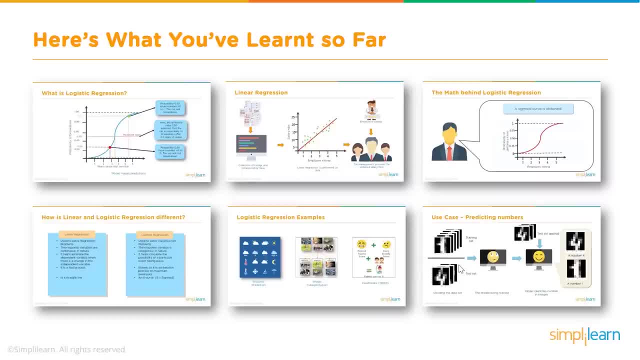 classification problems and then in the classification problems and then in the end we looked at the code to see how we end. we looked at the code to see how we end. we looked at the code to see how we can implement logistic regression to can implement logistic regression to. 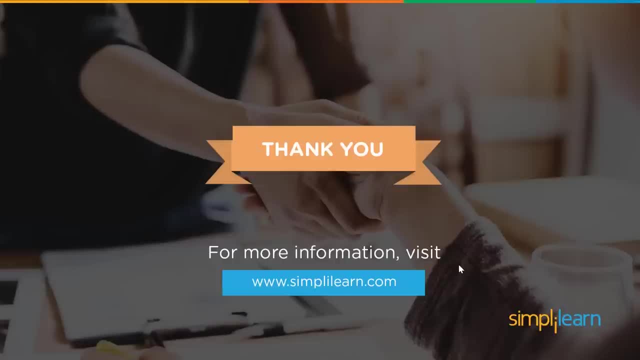 can implement logistic regression to train the model to identify images. with train the model to identify images. with train the model to identify images. with that, we come to the end of the session. that we come to the end of the session. that we come to the end of the session. thank you very much for watching this. 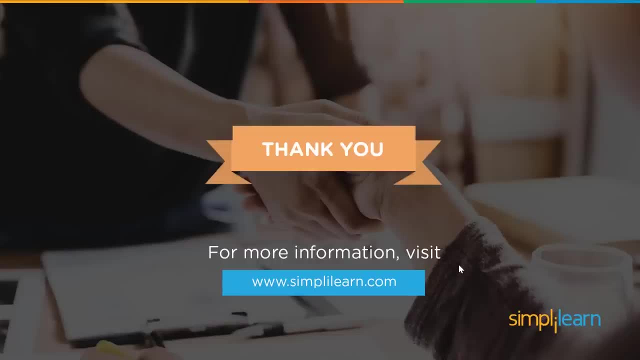 thank you very much for watching this. thank you very much for watching this video. for more information, visit us at video. for more information, visit us at video. for more information, visit us at wwwsimplylearncom and if you have any wwwsimplylearncom. and if you have any. 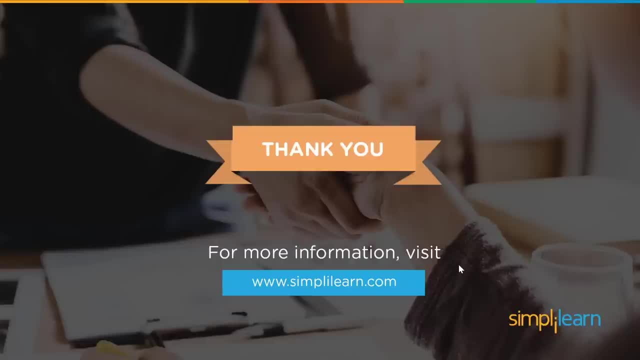 wwwsimplylearncom and if you have any further comments or feedback, please feel further comments or feedback. please feel further comments or feedback. please feel free to put your comments down below. free to put your comments down below. free to put your comments down below and thank you very much and you have a. 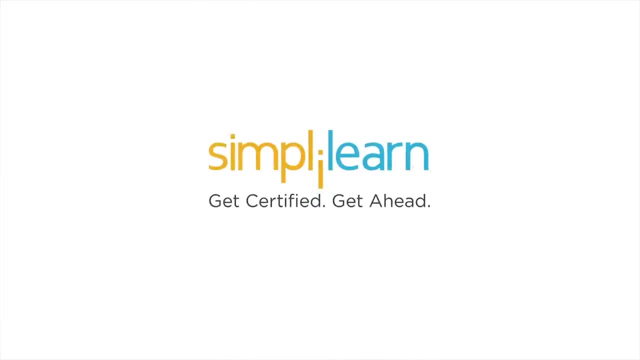 and thank you very much and you have a. and thank you very much and you have a great day hi there. if you like this video hi there. if you like this video hi there, if you like this video, subscribe to the simply learn youtube. subscribe to the simply learn youtube.